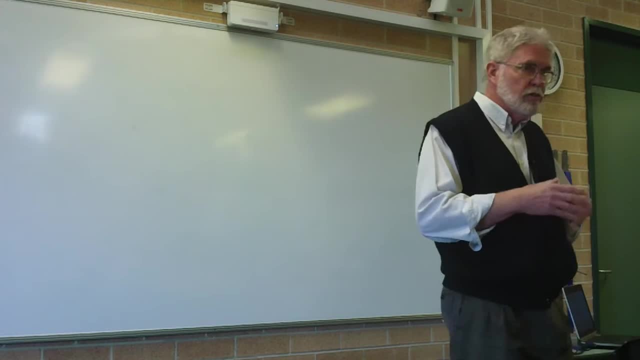 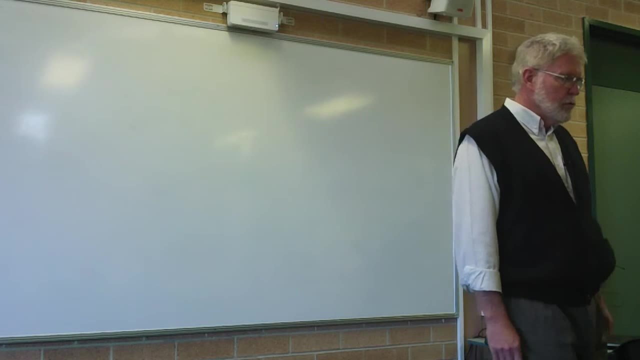 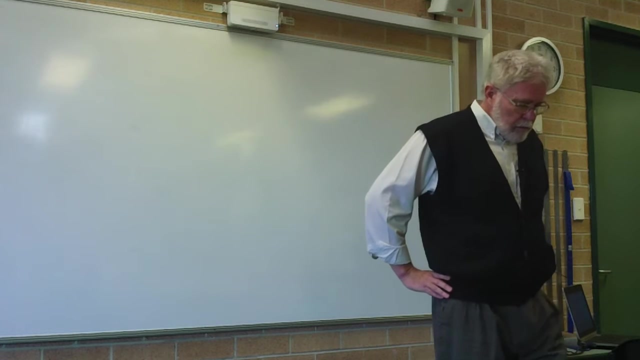 some of the idiosyncratic things that, as an engineering class, you need to be aware of. So there's history of aviation out there by the mile, and lots and lots of good videos with some good funny stuff and all that sort of gear. So what we're going to start with is: just what do you think would have been the first attempts of man to fly that were reasonably successful? by the way, Okay, Leonardo da Vinci did have some designs. No one has been able to replicate the designs into a position to fly. 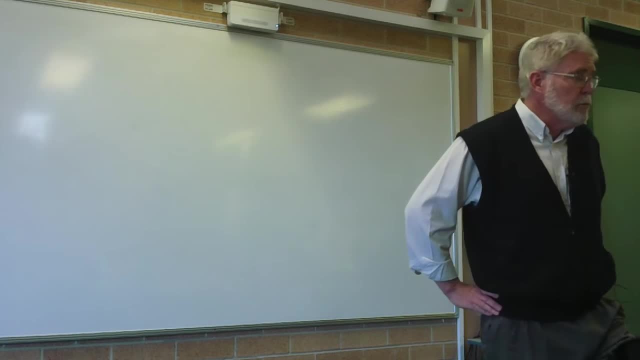 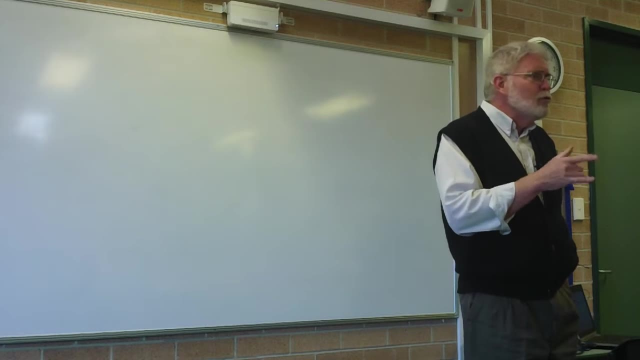 But they have. you been used to give guidelines to other people and we'll come to that in a moment. Leonardo da Vinci was in the what century About the 16th century? Oh, by the way, forgot. Did you do your homework? 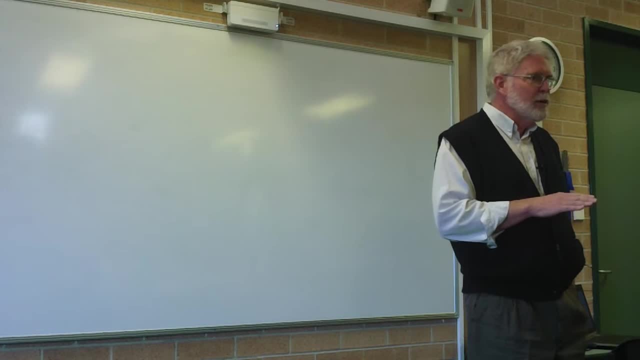 Which is tin and brass, Which one goes in brass and which one goes in. No, don't Google it, You're supposed to go away and find out. All right, Okay, What I tend to remember, just for that one. Now I know I'm digressing back, but just for this moment, because it was on the last video anyway. 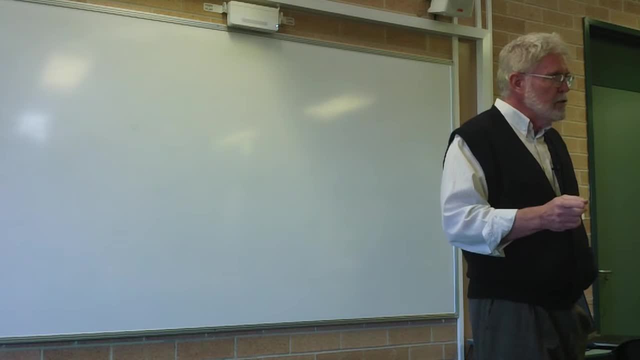 So brass and bronze are two very important copper alloys. right, Bronze comes first in the history of man because bronze is easy to alloy. And it's not easy to alloy. it's just that when you add something you could find readily, that's a product you find in lakes and sands, in lakes, Tin, tin deposits for reasonably easy to find. One of the cool things about this was it opening up supply lines. right, Yeah, Yeah, Yeah, Yeah, exactly, Yeah, Yeah. I mean okay, Okay, Okay, there's a question right there, Breaking a little bit of overs: an absolute, the initially interesting one. 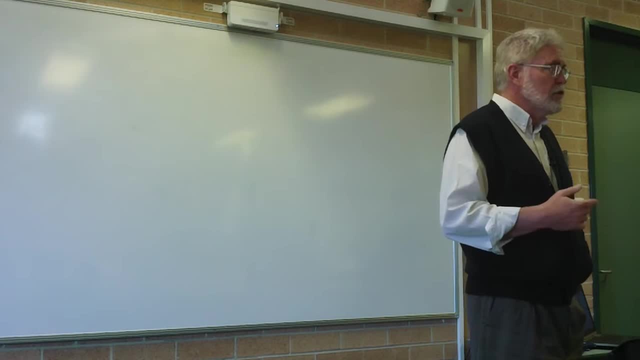 this was. it opened up trade routes because tin was prominently found in asia and the europeans wanted it and it was one of those things that the market across through asia was the the you'd hear about the silk road, but there may have just been as much money spent on transporting tin. 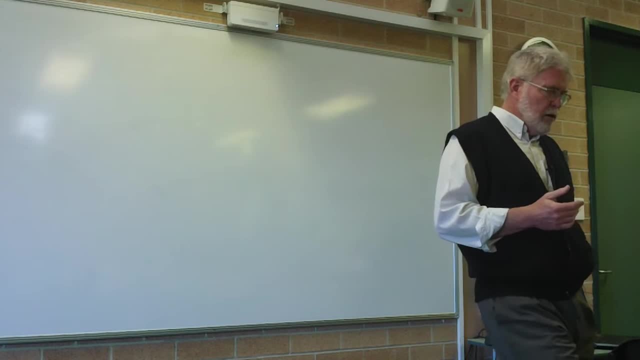 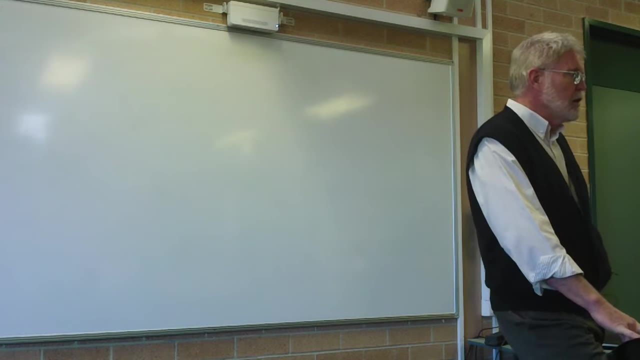 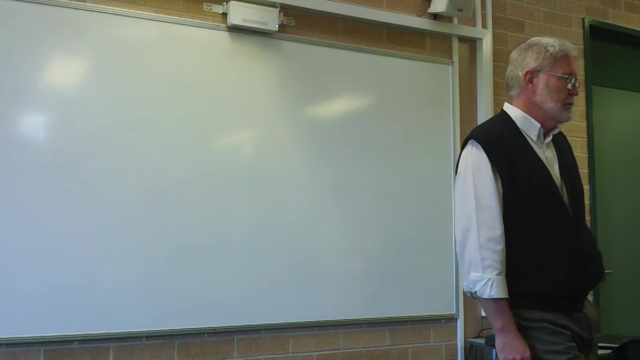 and getting tin into the mediterranean, um, anyway. so tin, tin, bronze is probably the easiest way to remember it. but remember the bronze age is when you go, you know it's an identity of a period of time based on the metal working that's being done. brass is zinc. now it gets a bit tricky because you 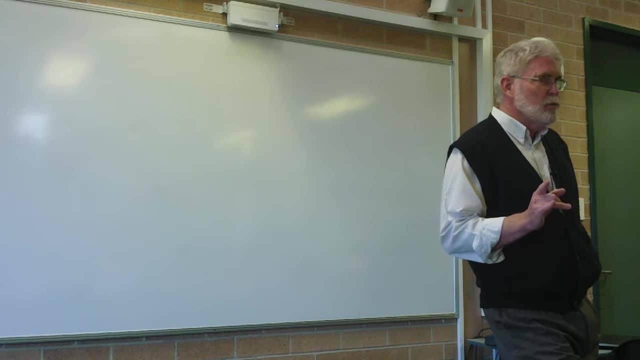 can alloy zinc and tin. if you have a predominant amount of zinc, it becomes a brass. if you put a predominant amount of tin in it, you can still have zinc in it and you call it a bronze. you can also add nickel and you get the copper and nickels and and you get all these ranges within it. so 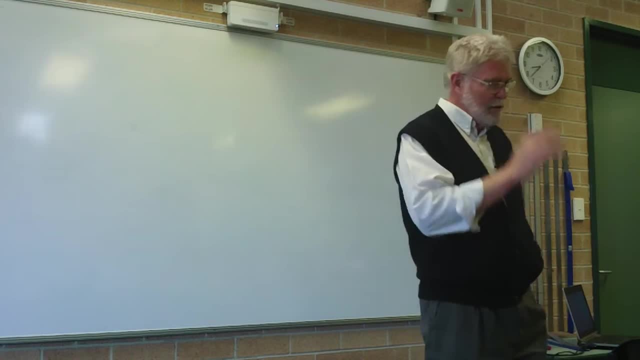 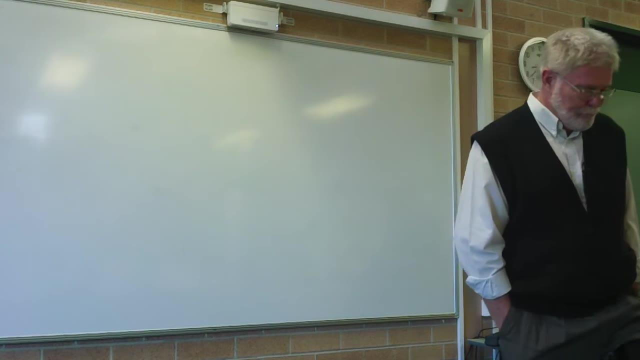 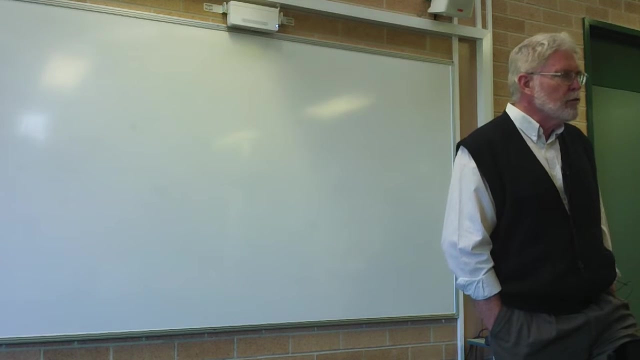 anyway, bottom line is for the answer to yesterday's question was: should have answered tin for bronze, zinc for brass. okay, remember that for next time. okay, back to aircraft, first flight. leonardo da vinci could have been one of the first people to think about flying in a very serious and 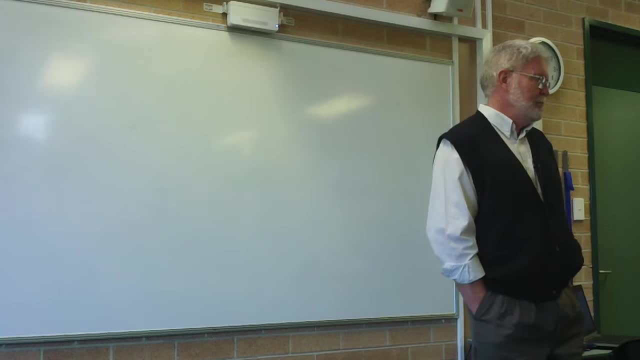 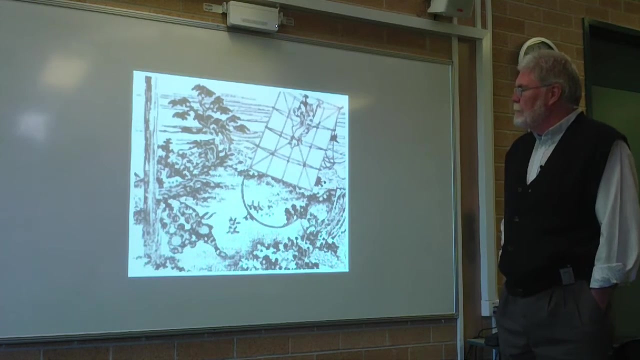 scientific way, but there were people doing this stuff before that, often not necessarily europeans. all right, let's have a look. you can't quite make this image out as well as you might, but it apparently is a painting on a wall. a painting on a wall in china. 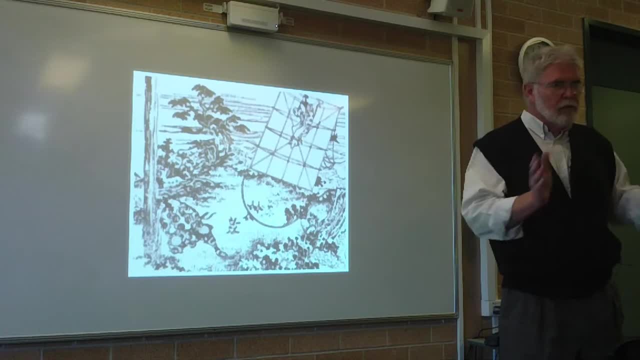 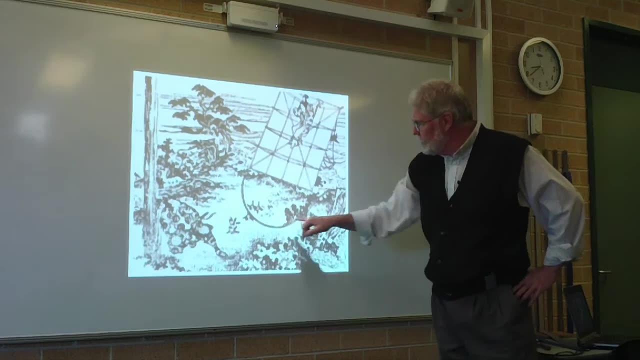 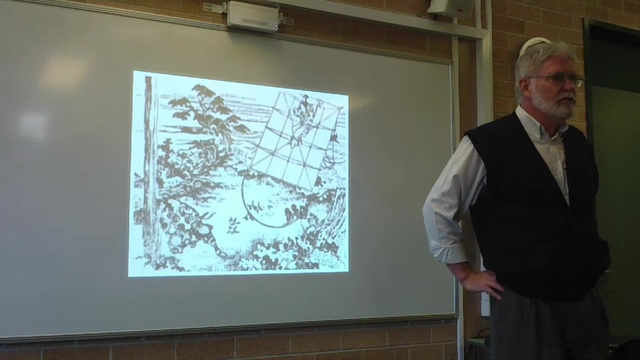 on a wall panel in a doorway- actually sliding door- of what appears to be a man strapped to a kite, tethered to the ground and quite considerably high up. now, whether or not this was very successful sounds very dangerous, but it's a very successful painting and it's a very successful painting and 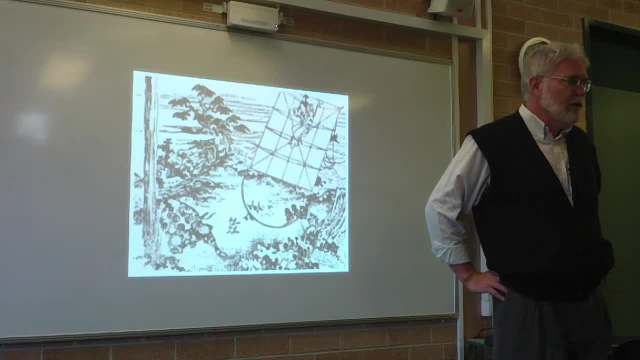 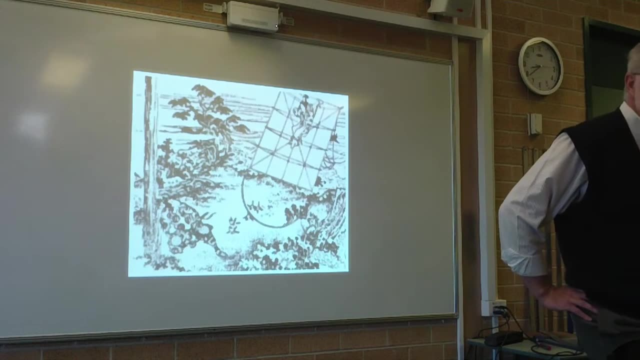 dangerous, because if you've ever flown a kite or if you fly- quite like i fly a kite often. they hit the ground at a rate of knots and if the wind isn't there for you, it's not going to work anyway, but it can be very- um, unpredictable. i'm not sure i want to be strapped to a kite, but just to go to. 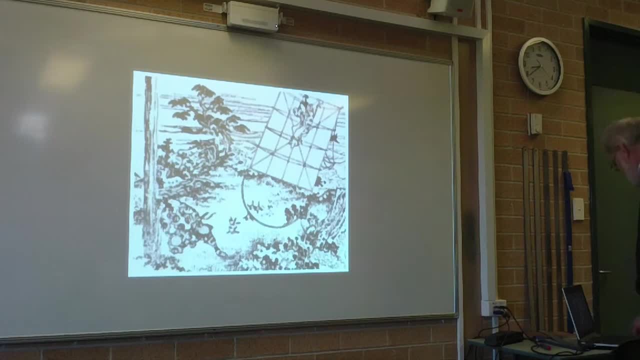 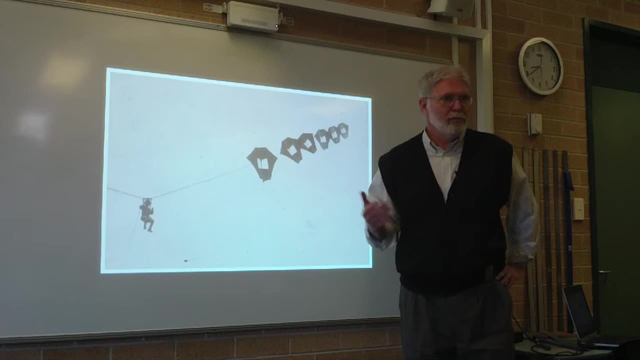 show that this idea isn't as dumb as it sounds, and we'll see what they used it for in a moment, but we think that maybe they were using it for military purposes. here is an example of a officer of something. well, i don't know he's an officer, but he's wearing one of those funny hats. 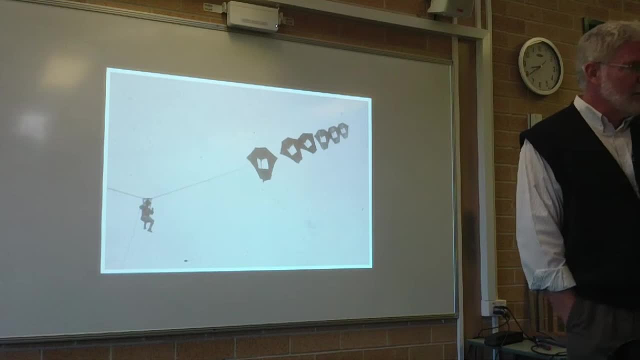 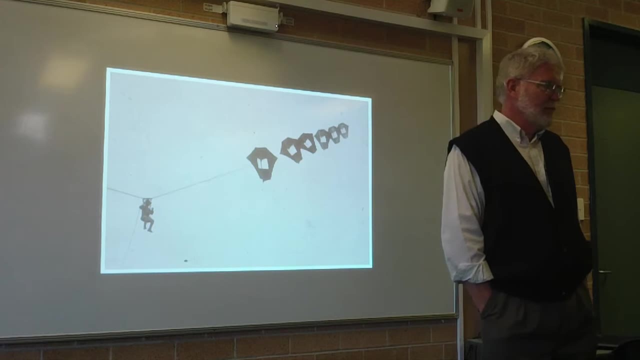 that they wore back in the turn of the century and i'd say he's american army or something like that, tethered to a whole bunch of tight kites. again doesn't sound like it's an extremely safe idea, but what we think they may have been doing with these sorts of things is getting a military. 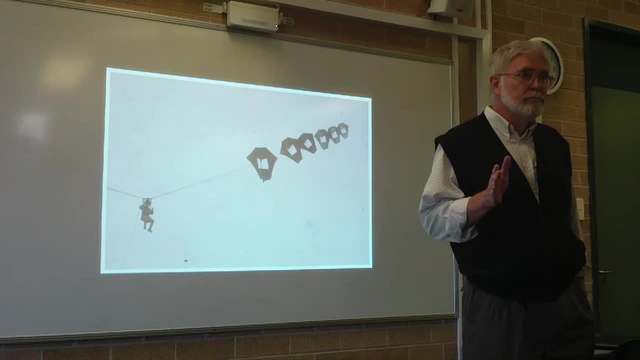 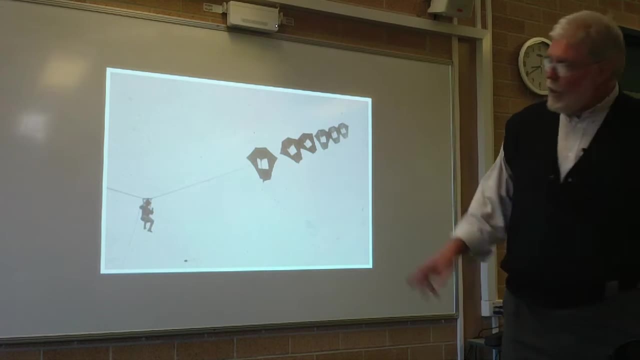 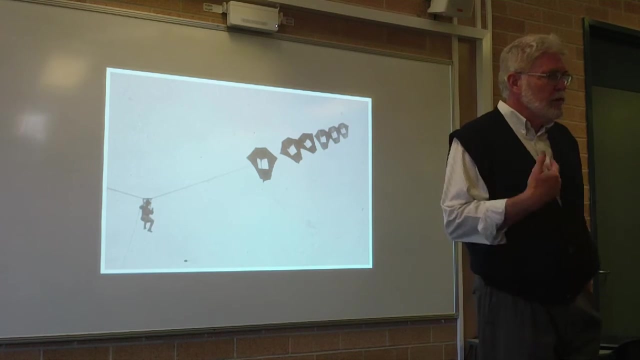 advantage by getting high enough to overlook an enemy army. so the chinese may have been doing it for that purpose. there's a reasonable suggestion. there is. that idea, by the way, pervades the history of flight for a very long time. we'll come to that in a moment. all right, so leonardo da vinci does do some designs. 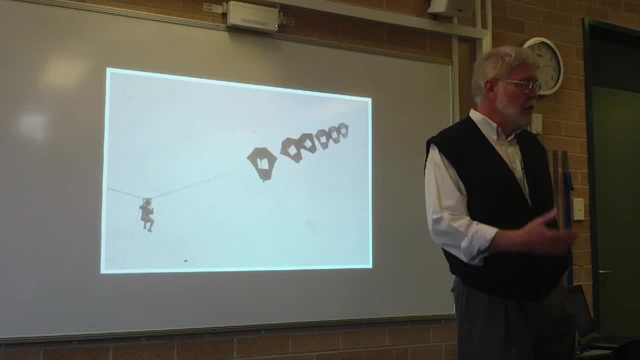 16th, 17th century, actually 15th, going into the 16th century, so that's a little bit early for what we're looking at next. what do you think the next big advance would have been? blighters could have been, yeah. now you're still thinking in terms of flight being oriented to wings. here's a kite. 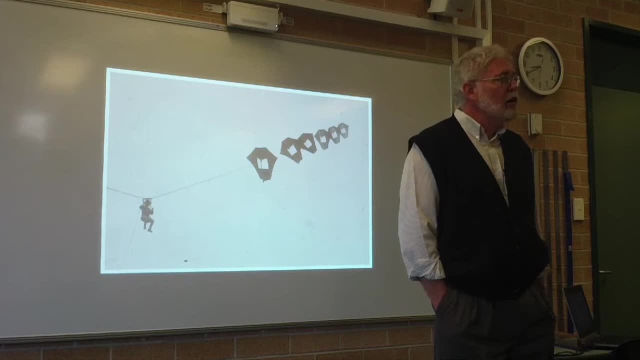 and flight is taking place. hot air balloons now. what do you mean by hot air balloons? now? what do you mean by hot air balloons? hot air balloons now. what do you mean by hot air balloons? what's the idea behind a balloon? in fact, we'll get a slide up. okay, so what? what's the advantage of hot air? hot air rises. why does hot air rise? because it has a lowered density, okay, so the volume that the air occupies, because it's being accelerated by heat, expands so that it is now less dense than the surrounding area, the air outside, so it is actually a fluid type situation, like water. 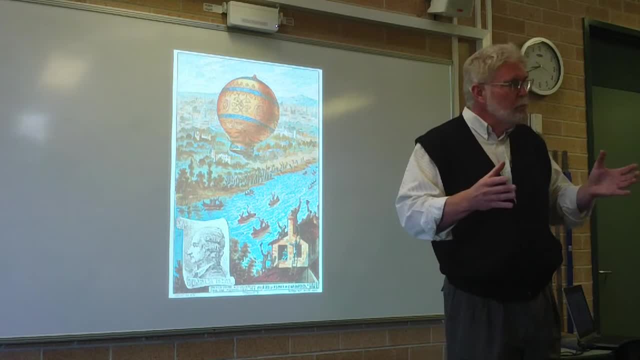 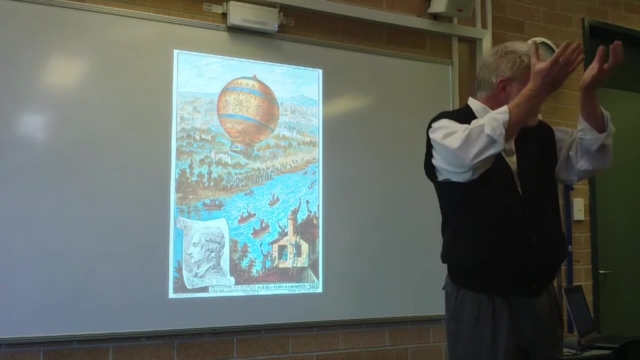 so if you can have something that displaces more than the weight of the water, it will float. same idea: if you can displace the volume of air and the air is lighter or there's less weight in that volume, then that volume will become buoyant. buoyant and will move, so heating the air underneath. now, what can you think would be actually have a 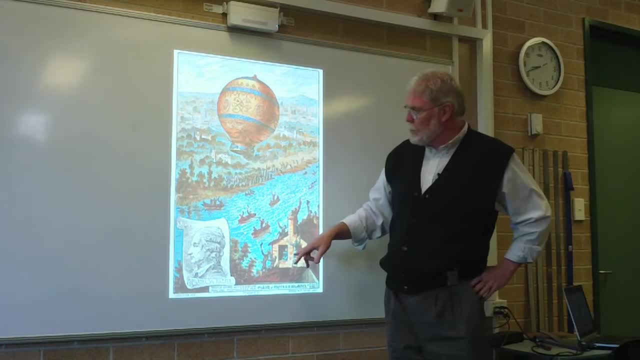 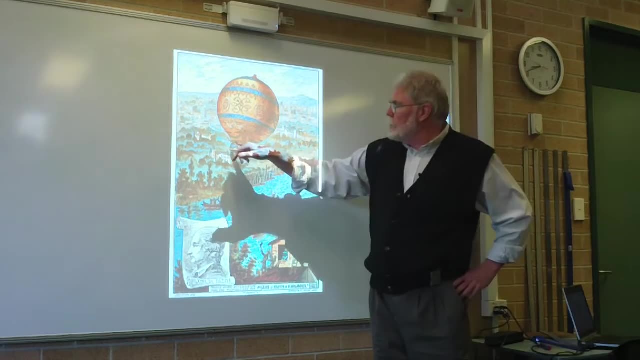 look at this. by the way, this is a picture of a postcard from a period in france where the guys were doing these experiments and actually quite good and the heights seem to be reasonable, everybody going, wow, look at this, but size of the ring around the outside that those guys are. 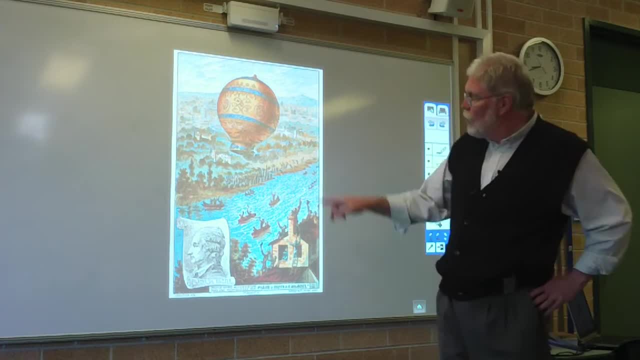 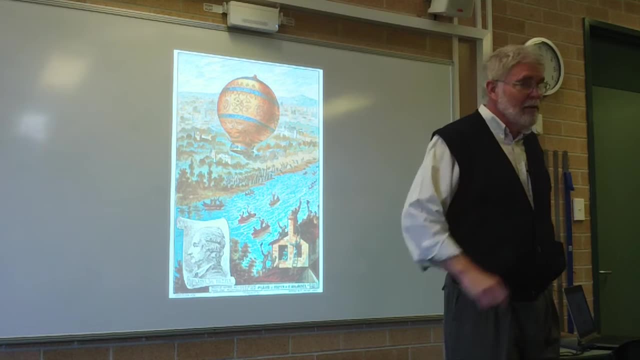 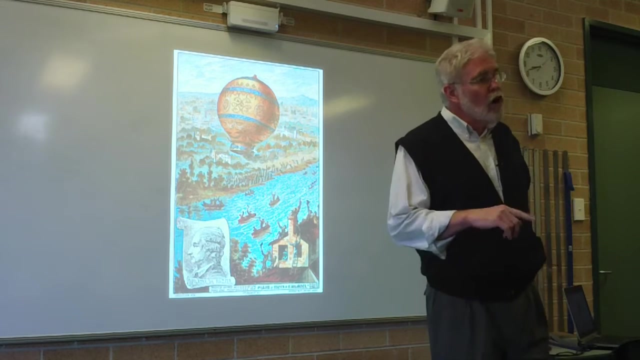 standing in this blue mark is not small. i mean, there's two guys there. by the way. you know, the fire is up underneath, which sounds a little bit dodgy, doesn't it right? and look at the angle he's on okay. so if you've got any sort of gust of wind that turn those things slightly, the fire that is. 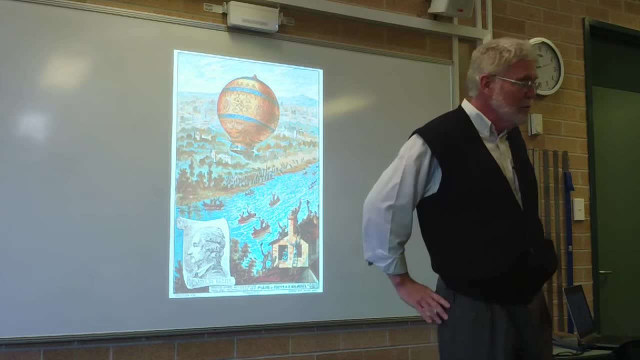 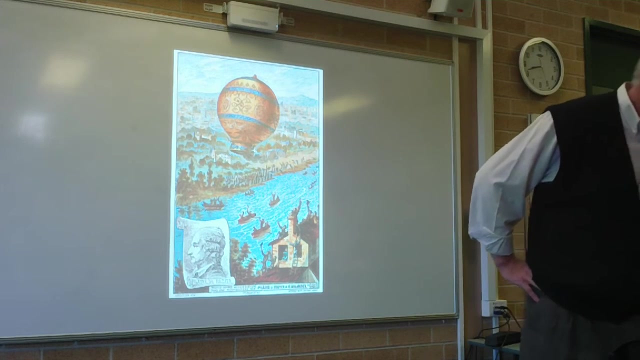 heating the air is likely to cause a problem. now, where do you think they got the idea for this? from? okay, good, asian paper candle there, absolutely. from what we can gather, you've heard the name marco polo, i presume supposedly one of these genoesian or. 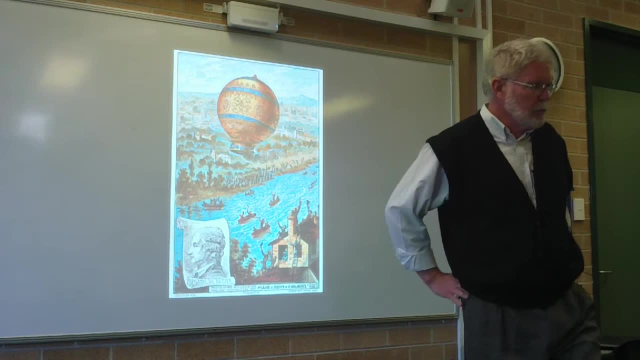 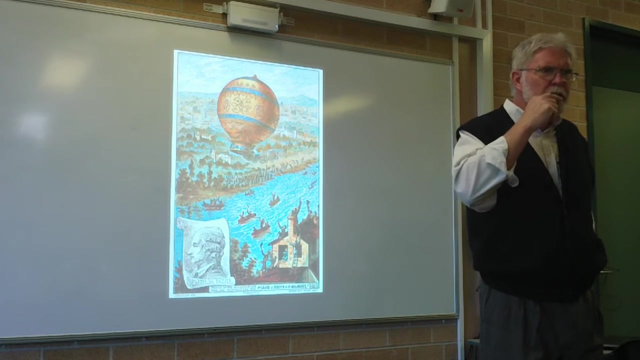 venetian, i can't remember now north italy guys who went and traveled over to china on on what probably was just really a business trip to try and drum up some work for transporting material back and stuff. he spent some time in the court. i think it was called a kublai car, wasn't it something like. 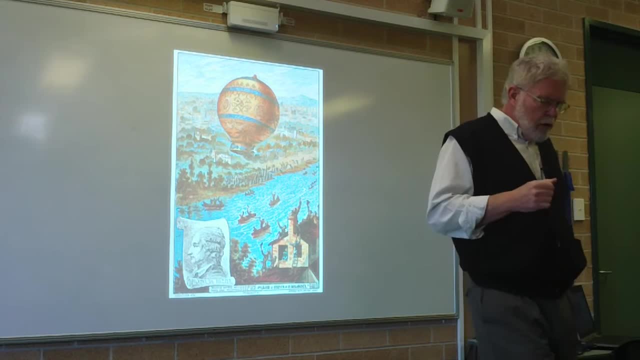 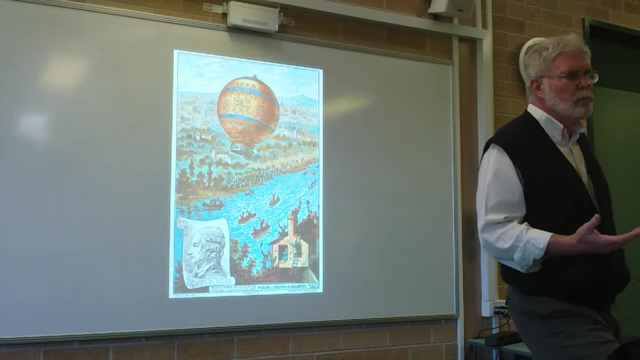 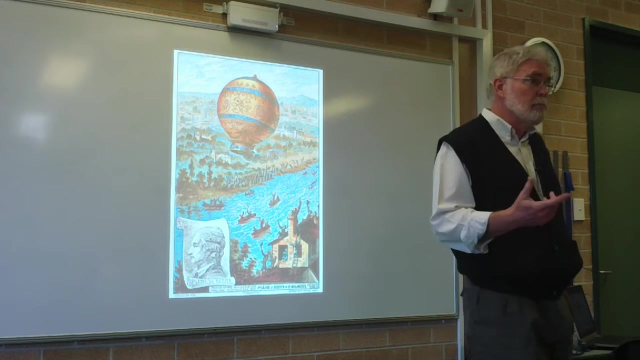 that sounds right, um, if it's not, google it. um, yeah, but that's the, the chinese emperor. he spent time there, which was unusual for a european to be allowed to do anyway, but in the process, what he determined was: he saw things, saw things. one of the big things he saw was the use of 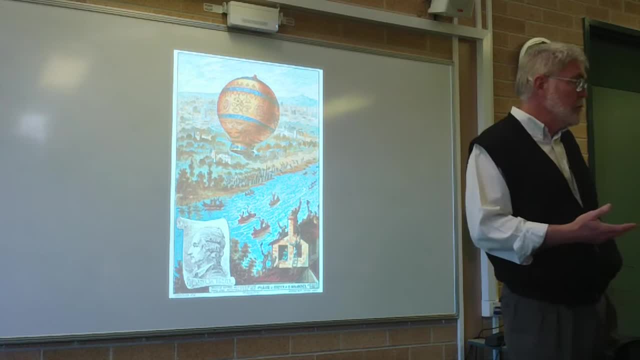 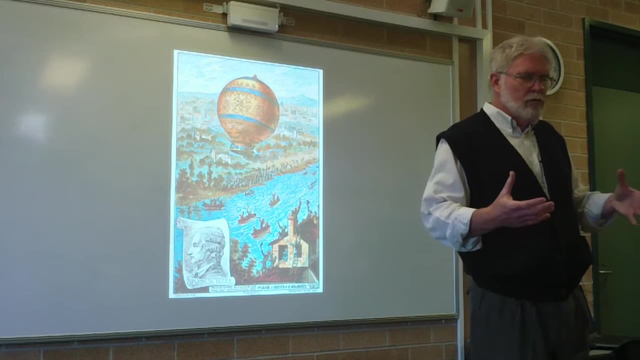 gunpowder for rocketry, um, which he would bring back into europe and that could cause. well, it changed europe overnight. uh, the sorts of things that that gunpowder would change, for example, would be the fact that, um, up until then, the nature of warfare in in europe would have been to build a fort, or 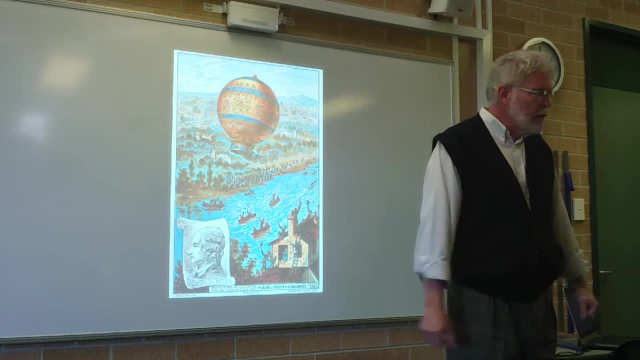 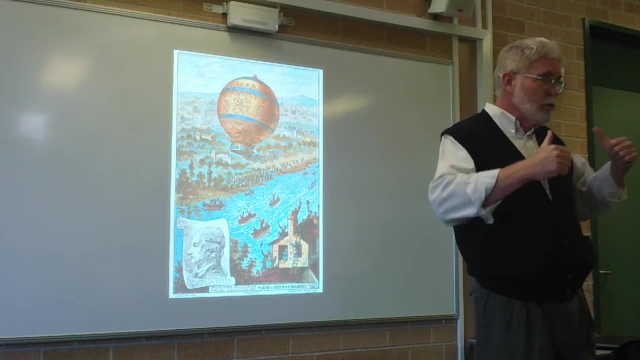 build a castle. um, when somebody comes to take over, you just pull the drawbridge up and everybody goes out, way out, wait out the siege. so if you've got more stuff inside than the guy outside, or you wait for the weather to change, uh, game of thrones. stannis didn't pick his timing really well. 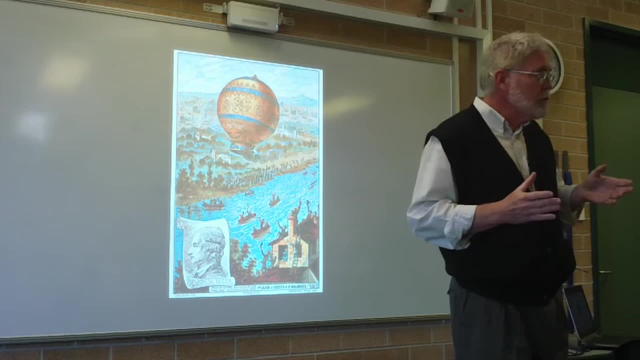 um, and so you know, you don't turn up and go on a siege when you've got no food. that doesn't work anyway. so that changed overnight because you couldn't go inside and pull the drawbridge up, because you just come along and blow the drawbridge up with a cannon. you blow up the 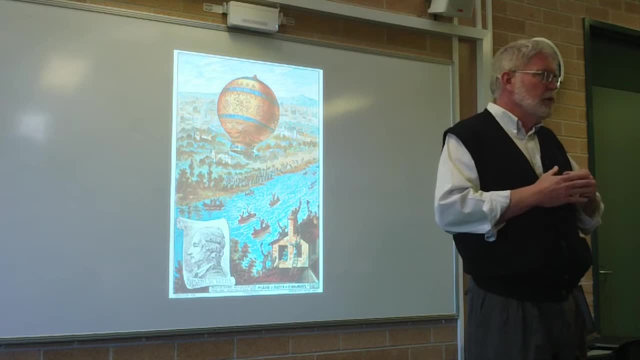 site change. it changed with um, the uh, the. around the time of the? uh crusades and the? uh, there was a lot of this siege stuff going on and the cannon was being brought in at that stage. anyway, that's going off track, but that's one of the other things that came out of. 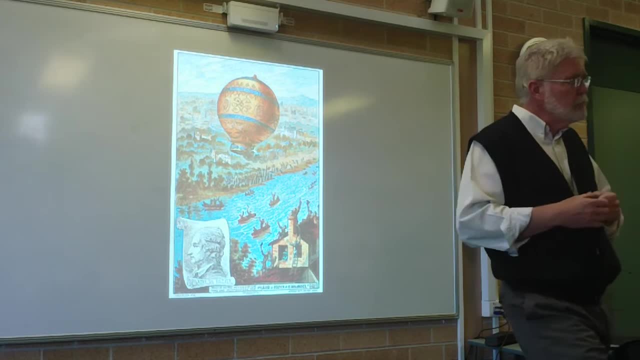 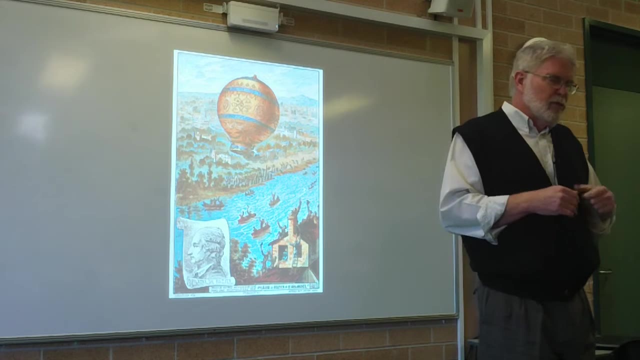 asia, probably also through the um, use of it by the muslims in the fighting with the christians and so on. anyway, uh, yeah, the crusades that weren't so holy. yeah, actually there's a whole bunch of stuff in history with that sort of thing. we got a lot out of that europe. 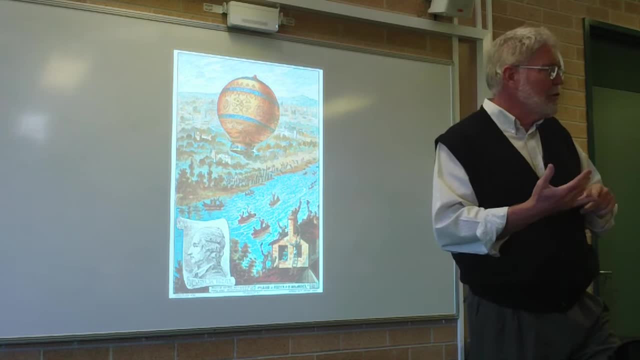 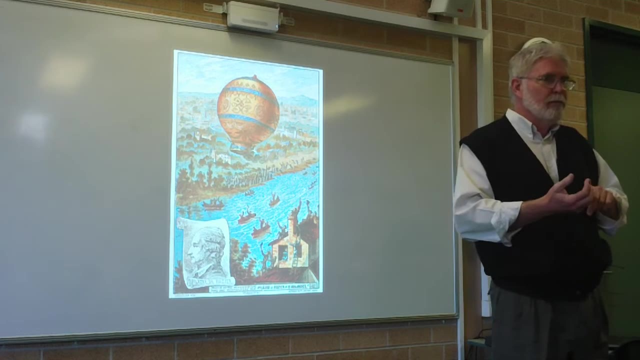 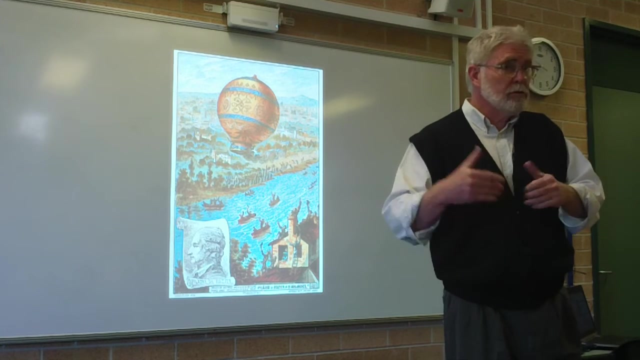 got numbers and we got science. um, you know, we got astronomy or astrology that turned into a better astronomy because the muslims were really good at all this stuff. um, algebra, yeah, yeah, absolutely. we call it the hindu arabic numerals because they're from that part of the world anyway. 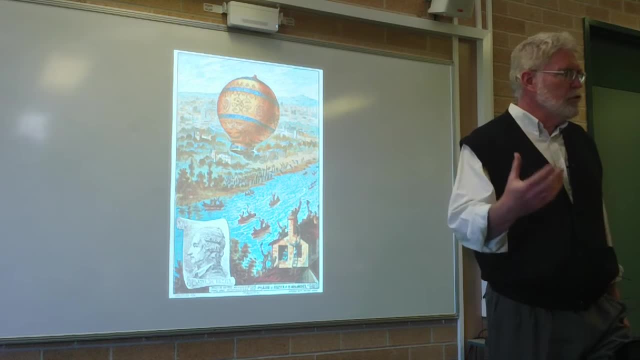 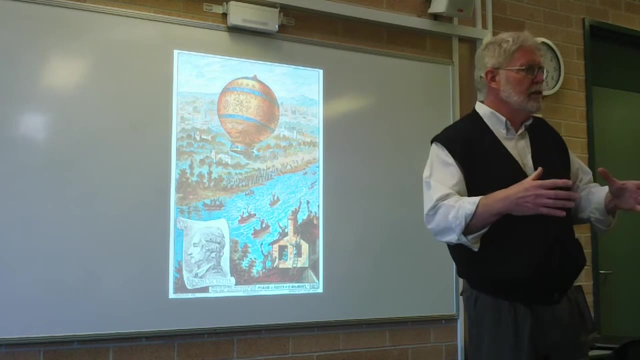 so we got the idea, perhaps through observing the kind of candle thing. now you have to wonder with the chinese sometimes is that if they had these brilliant ideas, why didn't they go further with them? just didn't seem to work. and it has to do with society and has to do with the way in which you 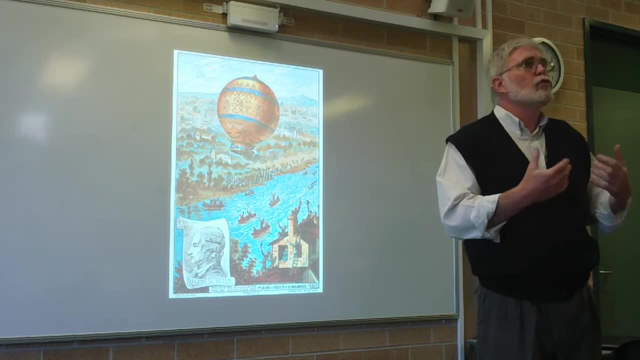 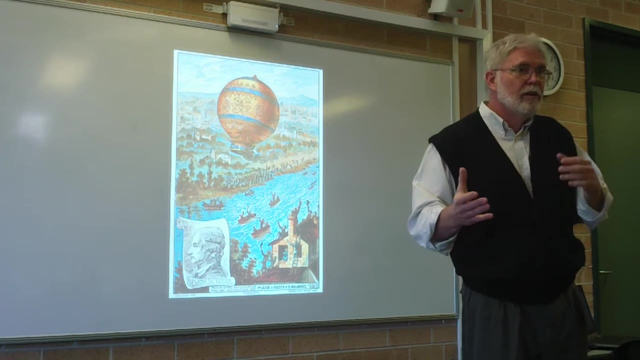 don't get your entrepreneurs, do not get benefit from being providing material for the emperor, the emperor gets it all. so you need a change of society. you need something like europe coming up, where if you've got a good idea and you can market it, then you get to go to the front of the line. 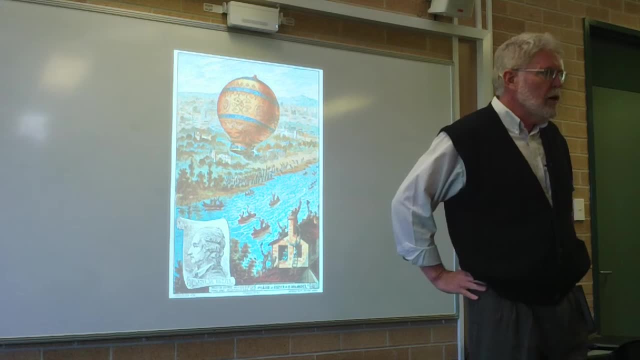 anyway. so hot air balloons- a bit dodgy bit, they work. we still use a variation of that now because if you've been down to canberra in the mornings in the winter and on those still mornings, you can see the balloons floating above canberra looking stunning. um, they're all hot air balloons, and at this. but 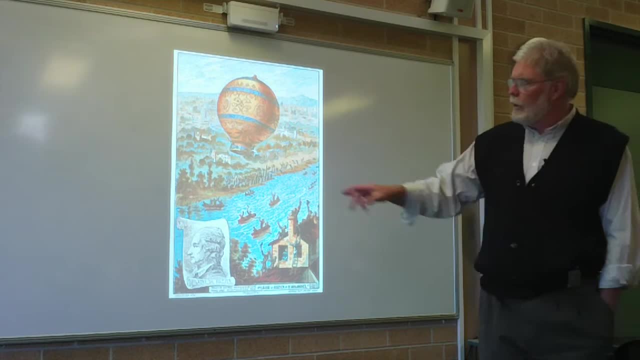 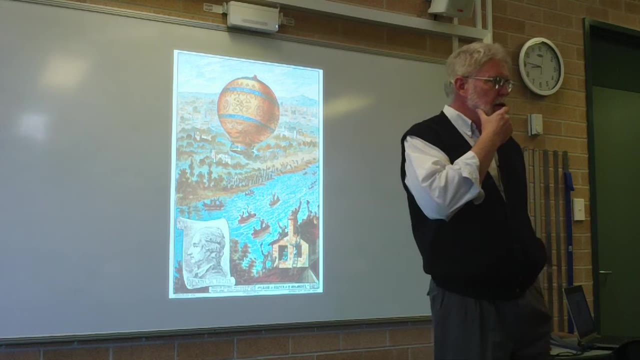 it's very controlled now because we can do it much better. we don't have a. they have to have a fire. they didn't have propane gas going here. all right, what do you think the next development might have been out of the balloons, it could be okay. helium is a good idea, but there's a problem. it takes a little bit more science now to get to. 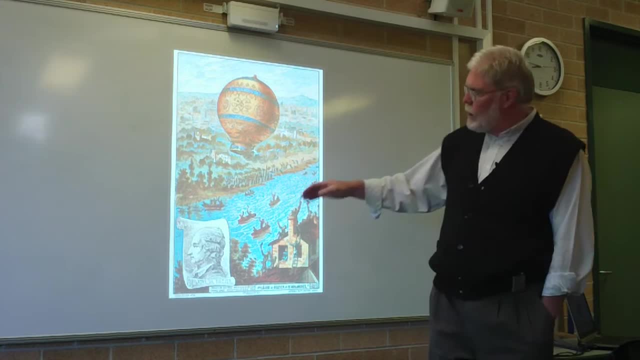 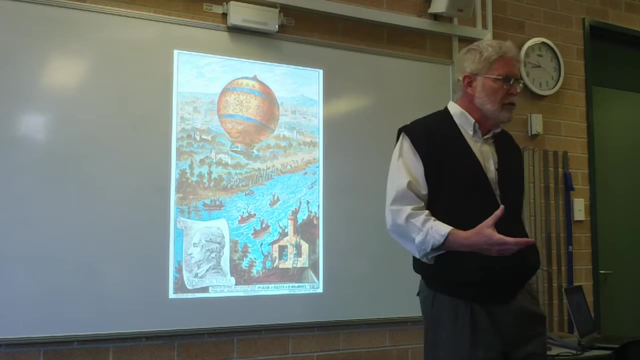 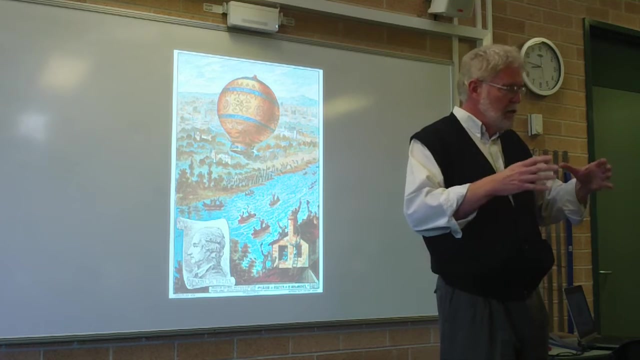 a place where we can start creating balloons. this is around the end of the the the 18th century, so six, the 1750s, 1770s. at the same time as that, what's going on in science? what sorts of things are happening? what sort of names do you think of associated with the late sixth, late 18th century? 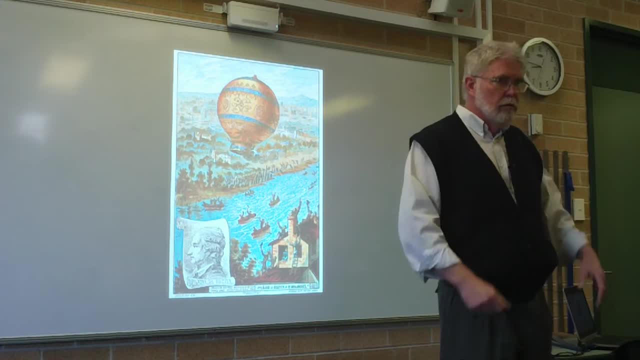 some famous names, guys with wigs, darwin's a little bit later. his grandfather was in this period, erasmus, and he was doing some work on that sort of stuff that darwin would pick up on, newton. yeah, what have we learned? who the guys we? 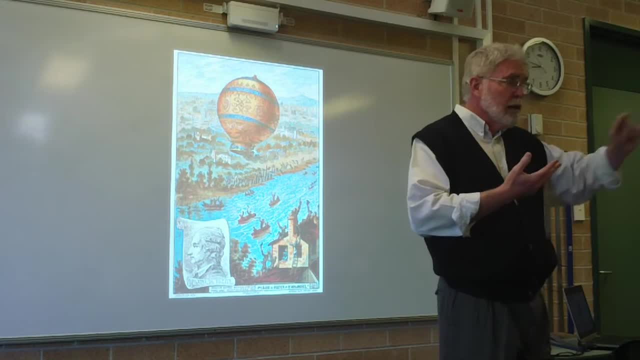 learned about with electricity. no, a little bit later he's. he's in the 1800s. uh, volta, from where we get volts, galvin, it's your running from where we get the galvanics series batteries were being looked at because we're working out that if you put two dissimilar metals- remember we 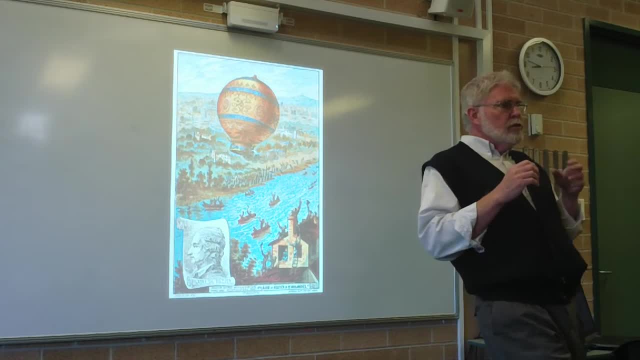 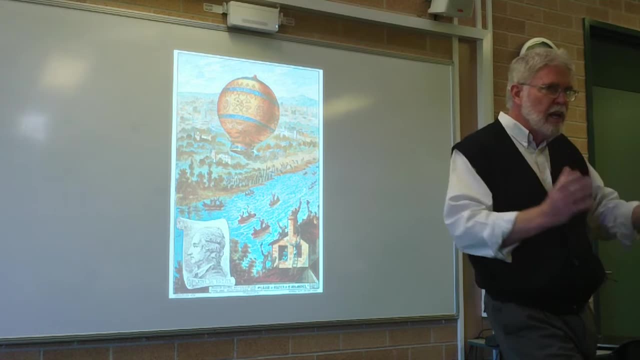 talked about this- in an electrolyte should get up a current and, as a result of the rebirth in science and guys like these guys, so and, and, and people who are looking at the chemistry that was going on, the what was, what's the nature of the world around them, they discovered a couple. 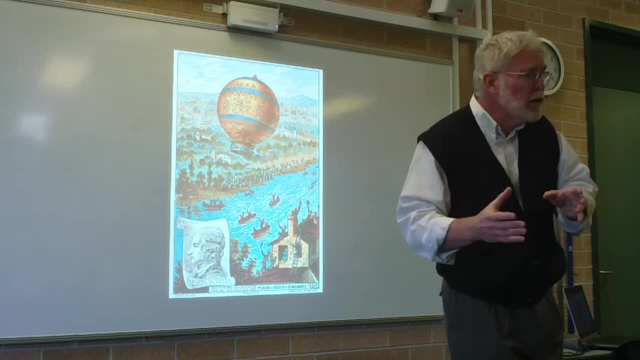 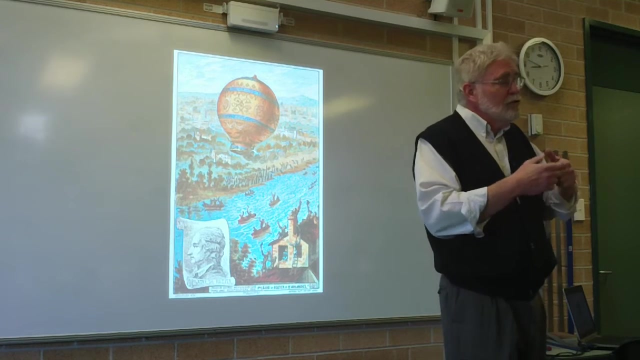 of things by accident, not by accident by experiment, but didn't? they were looking at one thing and found another. of the things they worked out was: if you pass a current through water, you can dissociate it. you can get the oxygen and hydrogen to come apart, all right. now there's a couple of things about. 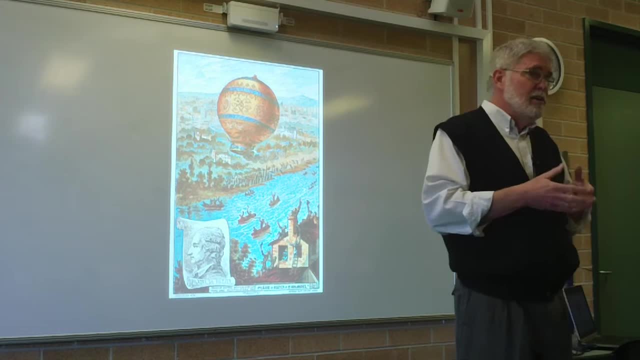 these lighter than air gases- okay, natural forming hydrogen, which you might get as a result of decay, and, close to it, methane. you know these very light gases. they don't tend to stick around down here with us. they are lighter than air, so they go up and out. they can actually reach the point where 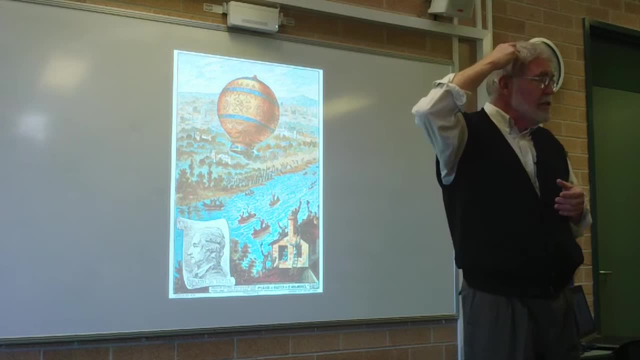 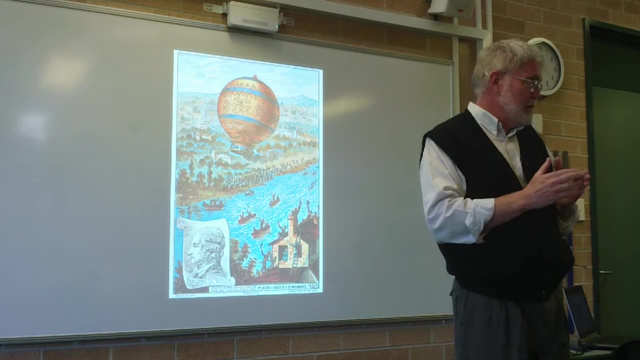 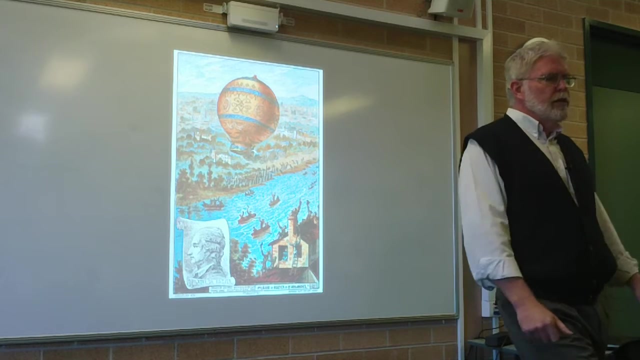 they are lost to space. and the one that's a classic for this is helium. now, helium was not discovered at this time, hydrogen was. now there's another character, a little russian guy. a little, he was a reasonable size, like then he. he was doing doing work in russia on genetics. 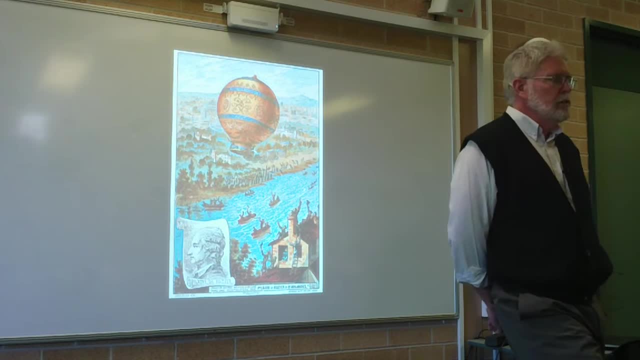 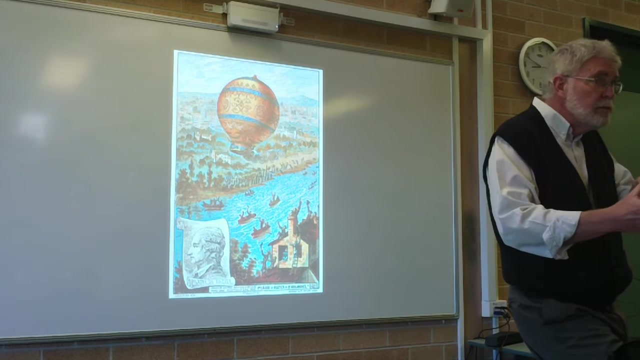 so you tutaj and he was looking at um, you know, coding and making up patterns and taxonomy for the plants and things, and he put his mind to why can't we do the same thing with elements? and he had, and there's a range of known elements, mendeleev, and he starts going already looking at what. 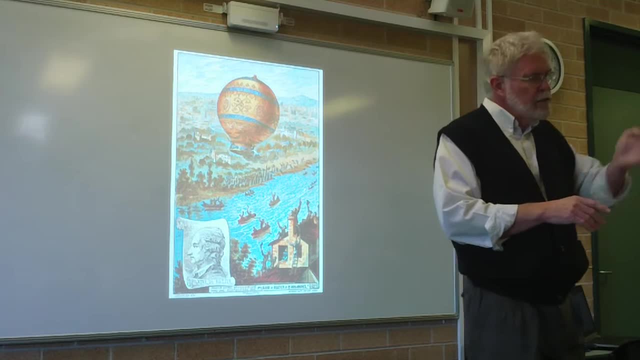 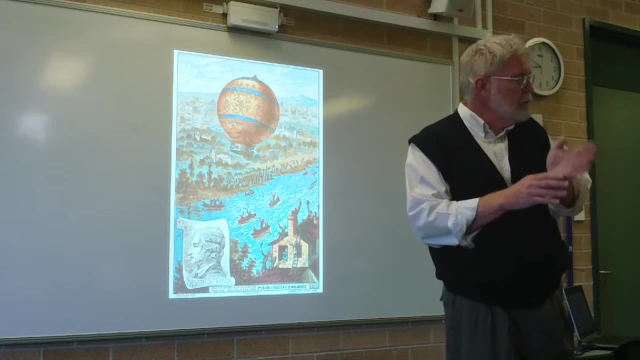 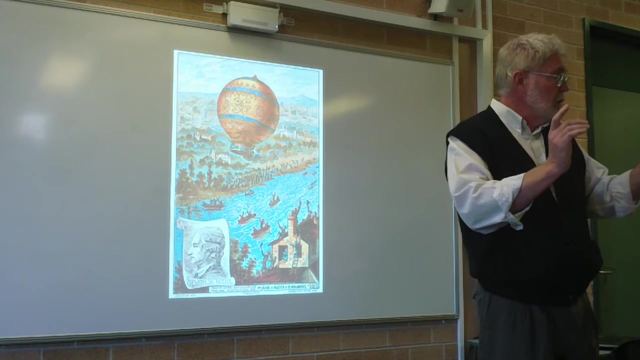 are the similarities between some of the materials, and he finds that as you start to look at their atomic weights, you can put them into groupings that are similar in and in properties. and he noticed that this repeated. first off, you know that he thought it repeated on a base of eight so he could move across and then it'd. 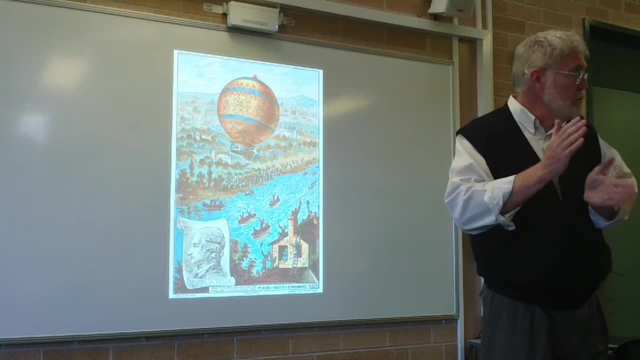 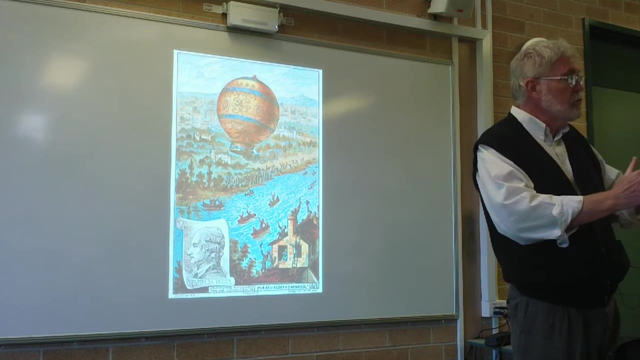 come back and start all over again, and he referred to them as periods in which these materials would act. the same related to the atomic weight, and of course they had to then move the table over a little bit to accommodate the things called the transition metals. and you, you start to see the pattern of what 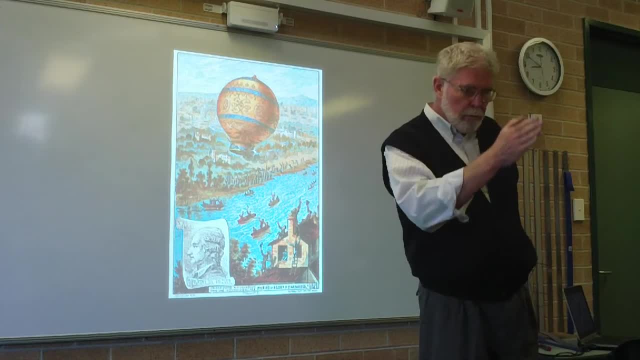 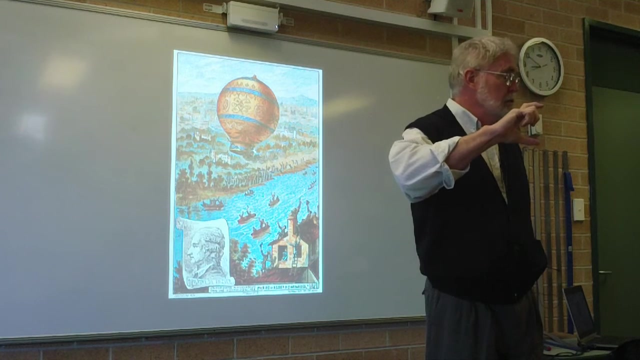 you know as the periodic table. but he'd noticed that this whole group of materials over on the right-hand side of his groupings that were inert. they were the kind of materials that would not combine with anything else and the top elements of them were natural gases and he found hydrogen worked on one side. 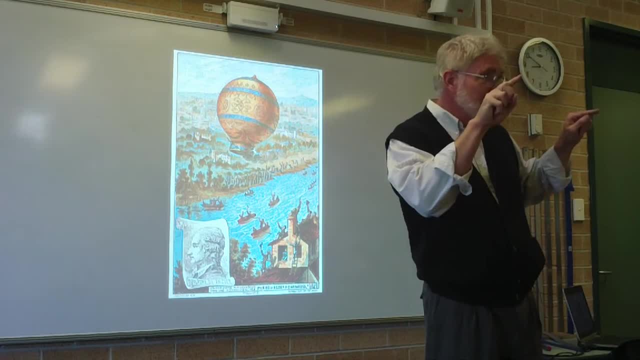 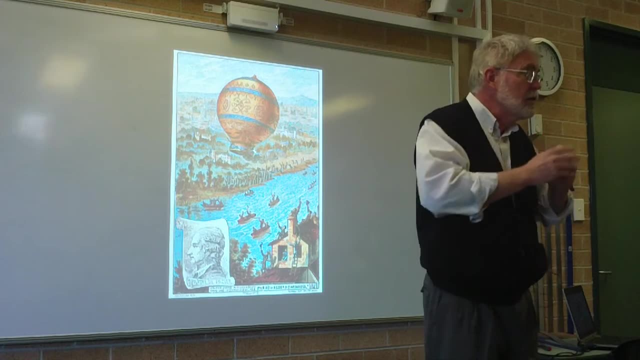 of the table, but there was a missing spot on the other side of the table, where he should be. there should be a gas that is inert, that is lighter than hydrogen, which was the first thing that he found. and then he looked at the other side of the table and he found that it was helium. so they started to 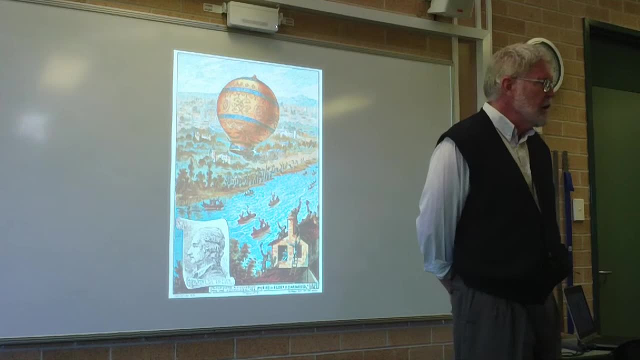 think in terms of, well, where what you find? helium? we can't find it in the atmosphere, because if it's lighter than air, it's gone. so they think maybe in mines, maybe in trapped areas within mines, where it hasn't actually got to the surface yet. and that's exactly what happened. they started to look for it and 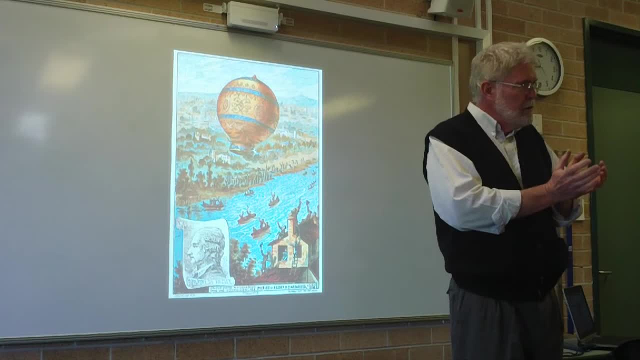 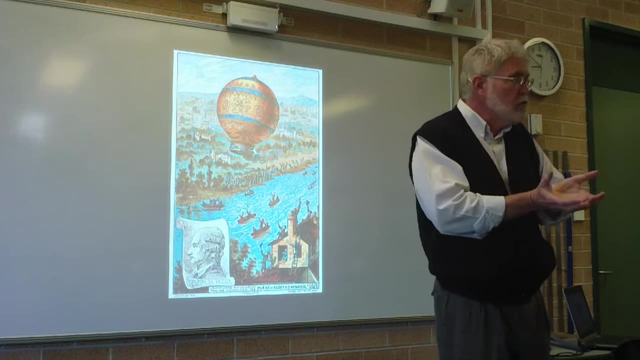 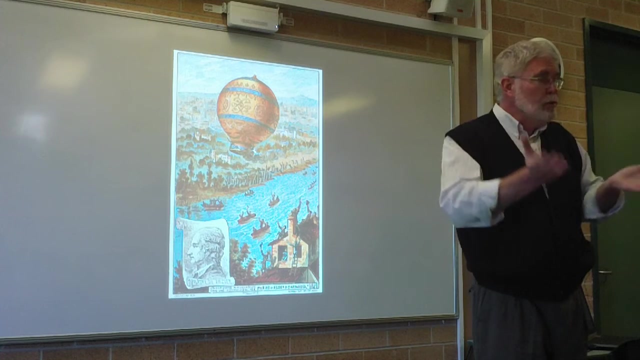 found it. but in the meantime they had worked out that if you put hydrogen in a container it's lighter than air. it displaces more than the volume that's around it, so it floats, and so you get your normal hydrogen balloons- now hot air balloons. you can control by turning the heat on and off. here hydrogen. balloons you've got to control by releasing weight to go up and releasing hydrogen to go down, so it's limited in in flight times too. the other thing about balloons is you really can't control where you're going because you're relying on the wind, so ballooning became a matter of climbing to an altitude. 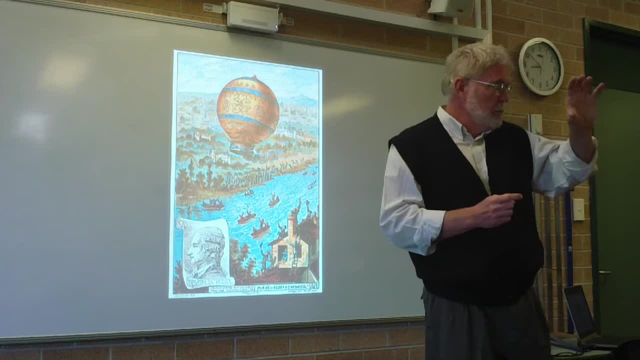 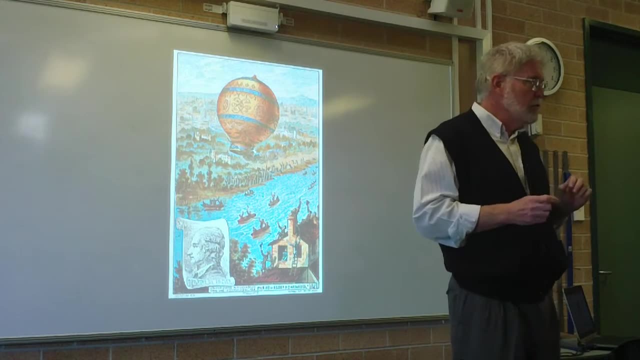 where you found a wind going the direction you wanted to go and going with it. now, if you've only got a limited amount of sandbags to throw out and a little amount of gas to let go, you sort of got to be really careful about how you do this if you want to go any long distance. so the first uses of balloons. 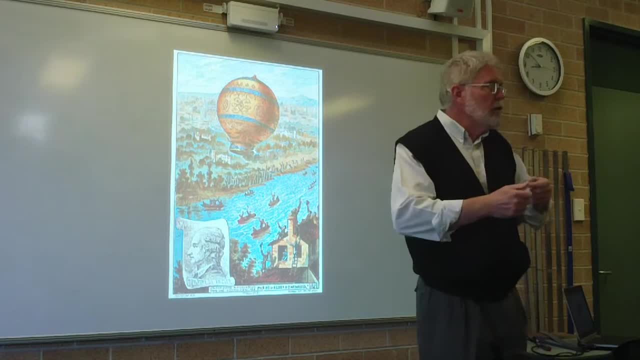 were tethered, so you just tied them to a rope so the guy could be pulled down or lifted up, right, whether it was hydrogen or helium. helium comes later, because hydrogen has a problem, and we'll talk about that in a moment, when we get to Zeppelin's and stuff. 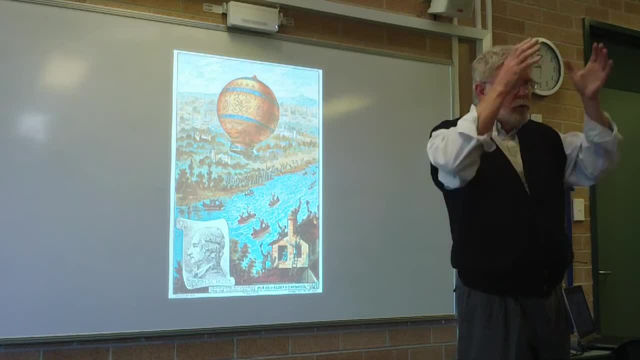 then you use them as a site, a place for observing military activity. one of the classic places where this came into its for was the American Civil War, because they use balloons on both sides to be able to observe opposite sides for gunnery, so you could target your gunnery. quite a few battles that were fought. 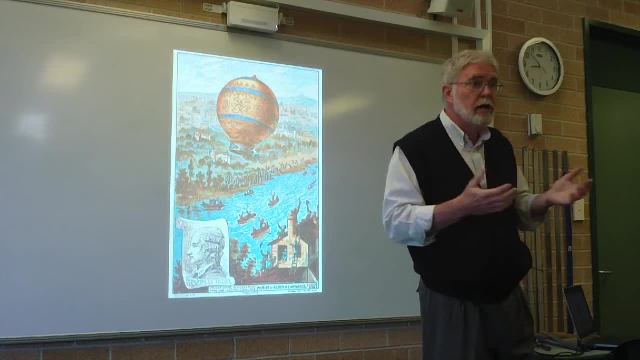 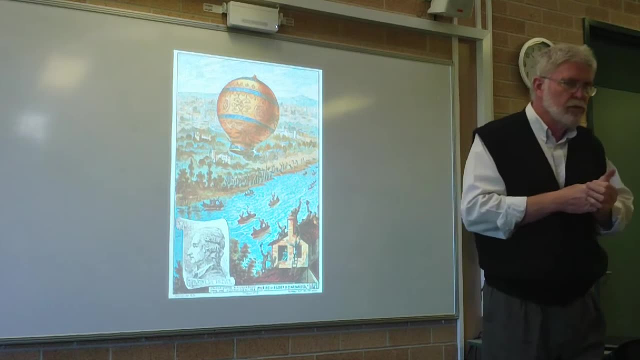 during the American Civil War relied on the fact that the Union Army had better ballooning than they could get in the south and had better observation, and that gave them an advantage, advantage not only the fact that they can make more stuff than the south, and so on, anyway. so 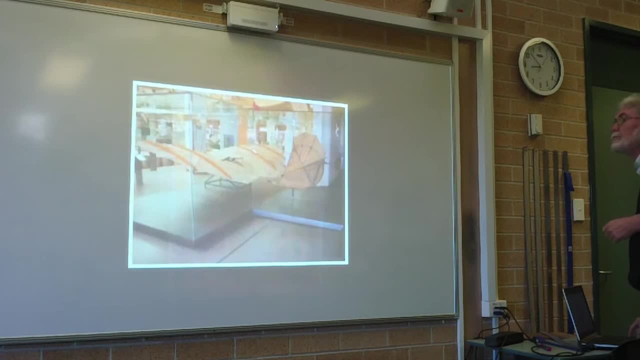 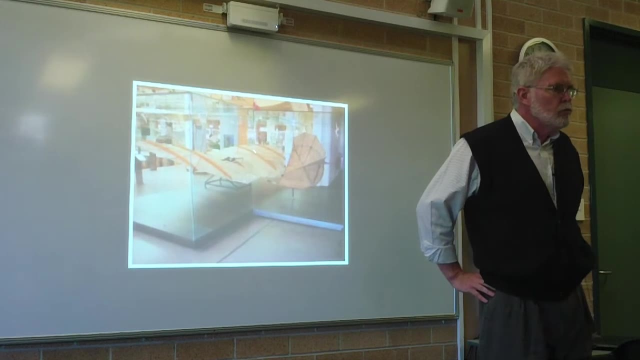 balloons. now let's look on a bit. middle of the 1800s, a couple of people started putting their mind to some of the ideas that they referred to back to da vinci, because his drawings look very similar to this one. this is by um, a fellow, a german guy, lilienthal um, and what he did was he. 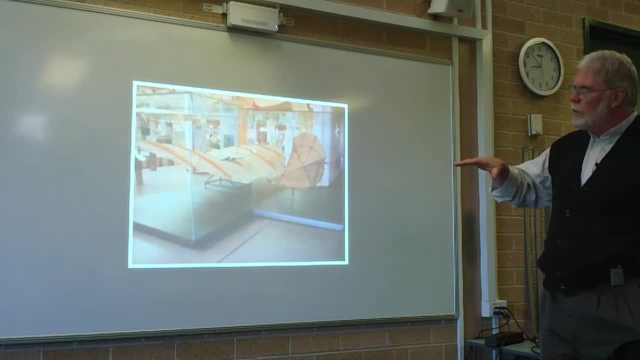 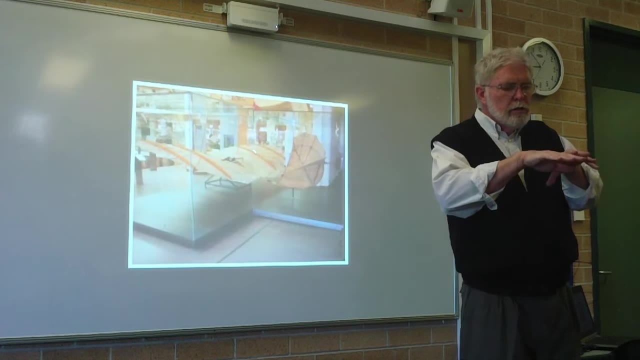 basically worked out that by looking at birds wings and looking at the shapes that the the birds did when they spread their feathers out. so the feathers are really interesting because what they do is that they create a shape that traps air but also allows for another property to take. 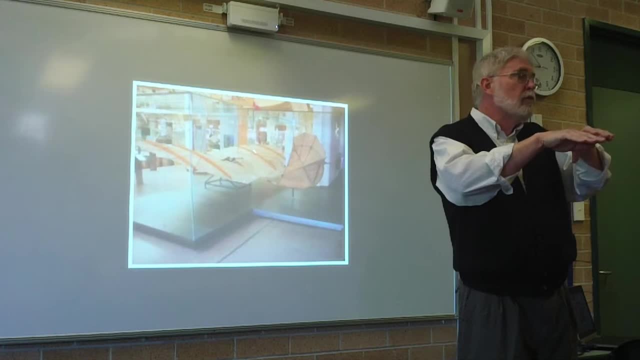 place which, as you're moving through the air, you now have an aerofoil situation coming up and we'll have a look at this in a moment when i draw it up on the board. but there's a principle that is here but took a while for them. 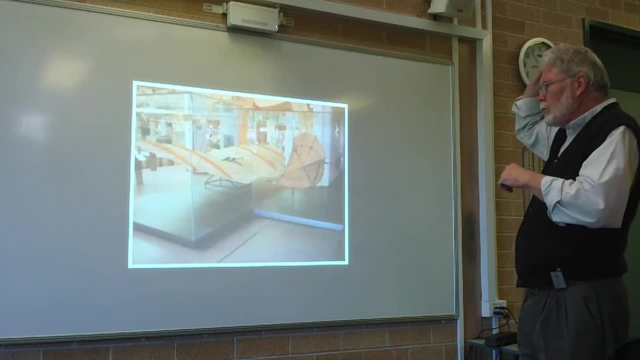 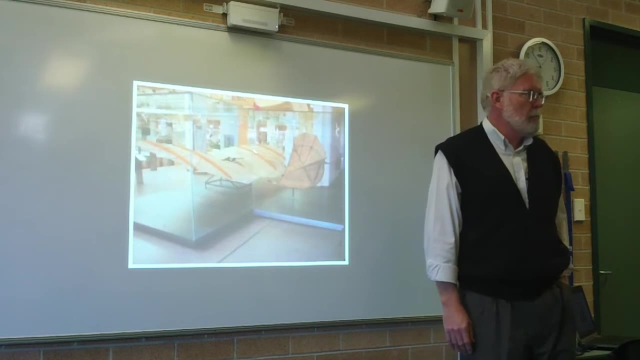 to actually determine what the principle was. so lilienthal just sort of said: well, why don't i build something that looks like a bird? and really what he has here is a slightly glorified hang glider. now, unfortunately for this gentleman, he was very successful at this and started showing. 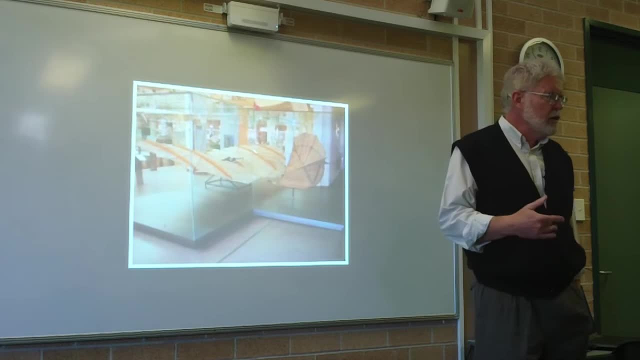 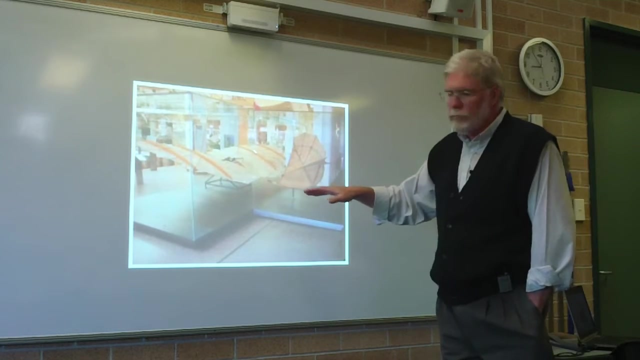 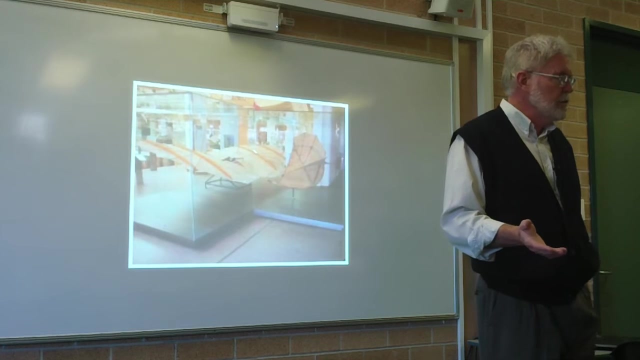 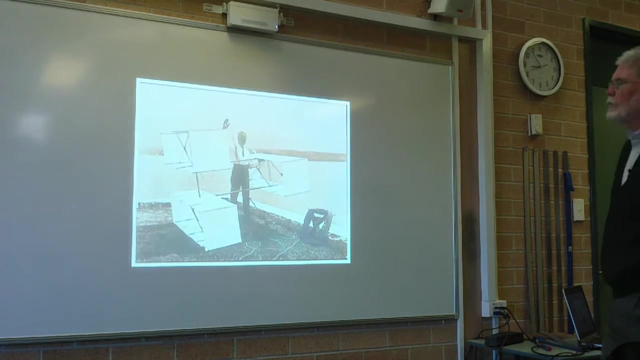 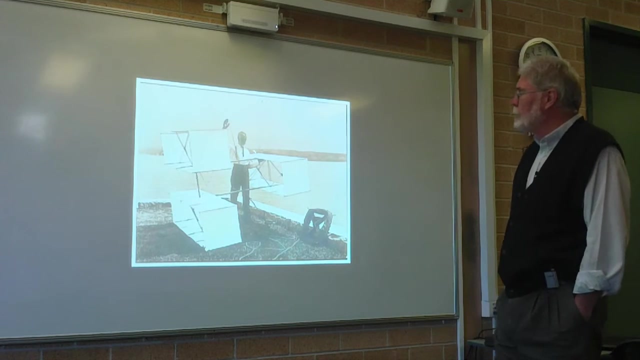 off two thousand flights or something. two and a half thousand flights he did successfully, but the last one wasn't, so he got killed flying. yeah, well, you don't tend to fly after the last one, especially if you're dead, so, but people paid attention to it and they thought this was pretty cool because he did manage to do it quite, quite successfully. very often it's a bit like hang gliding, now it's. it's a dodgy sport at the best of times. so you know you take all the risks when you do that. another one. anybody know who this guy- right, he's aussie, and this is actually a point piper i believe in in sydney at one stage, but he used to do the same stuff here just off seven mile beach. 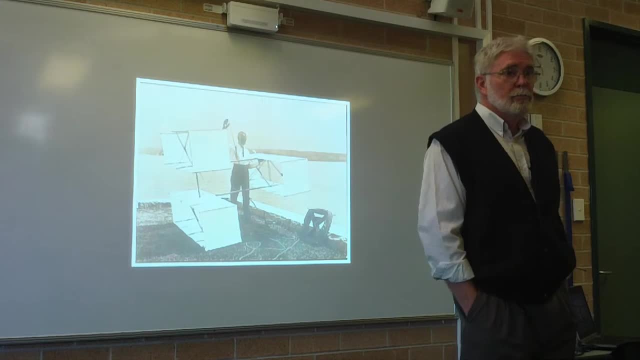 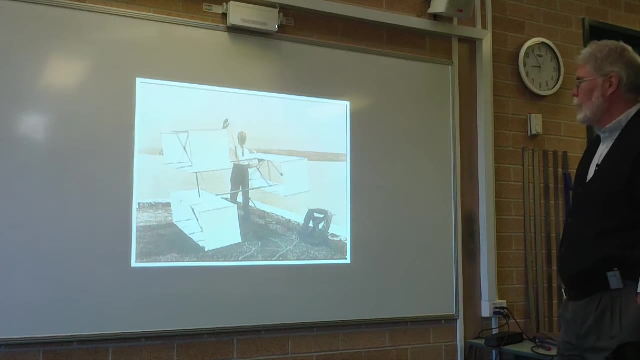 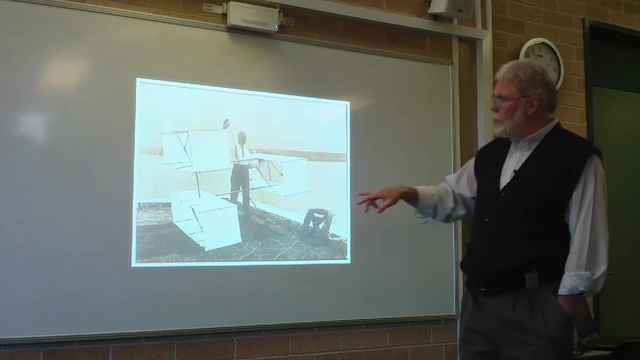 jiroa. top of the headlands there there's a park, hargrave, yeah, he's aussie, great edwin hargrave. now hargrave was looking, going back to the idea of the chinese and stuff, looking at kites and and box structures and and do you notice something slightly familiar? 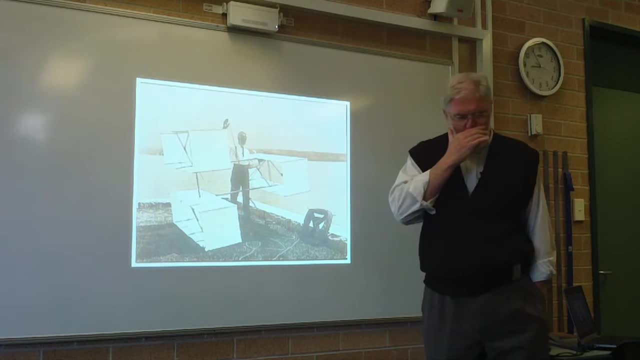 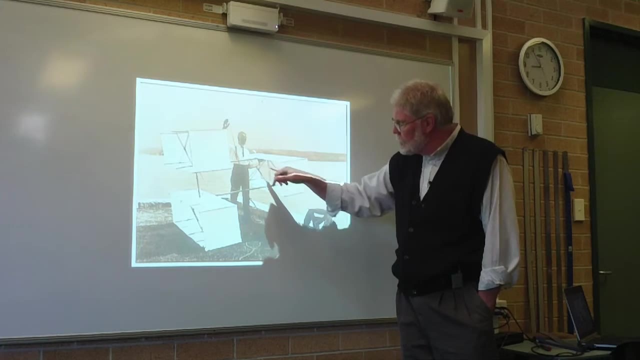 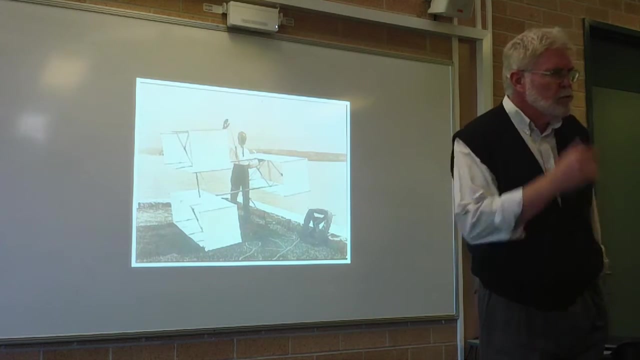 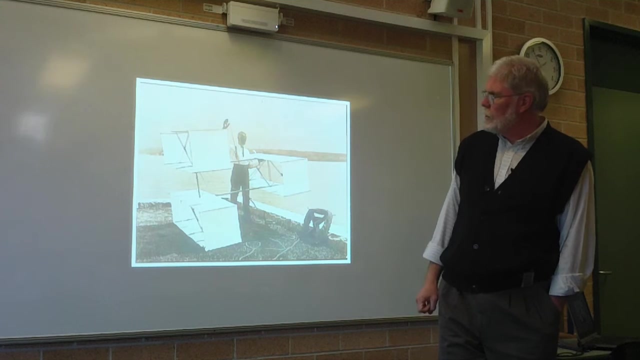 about this. if you don't, you'll see it in a moment. things that edward, that hargrave, did, that were to later become very important in flight, are the very thin spars, the cross members and the tightening with the wires. all right now, what's all? what else is happening in the 1700s, the late 1700s actually, this is a bit late. he's a bit of an older gentleman here. i believe this photo was taken early in the 19th, in the 20th century. 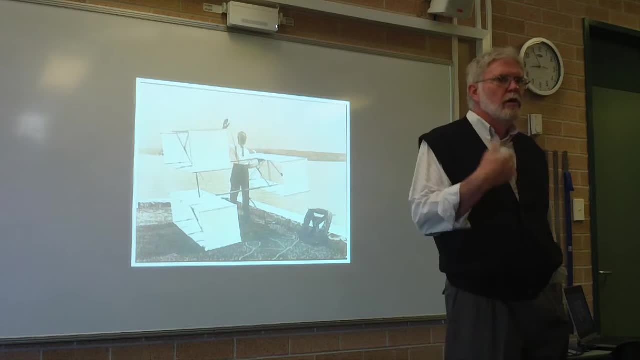 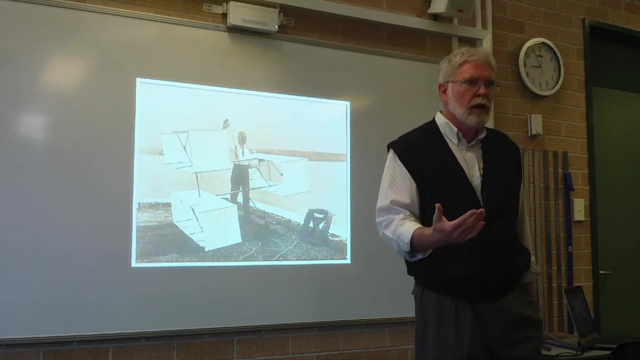 um, but by then he had a reputation, and that's why he's a photograph late 1700s, late 1800s, sorry, 1900s, 1960, 1970. where am i go back? 1860, 1870, what have we already looked at? that was happening in transportation for. 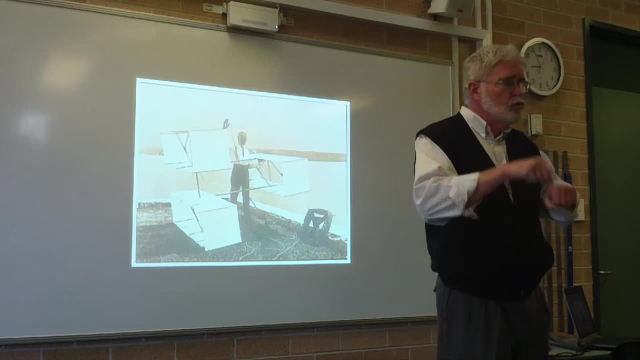 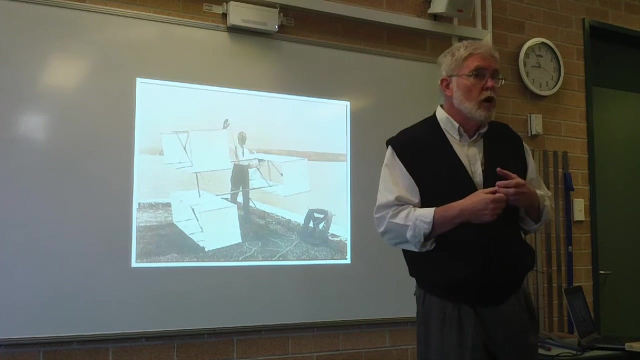 people back then, something that we- you- ride on bicycles, right. so bicycles were starting to come on board. now there's a whole lot of things about bicycles that are important. you start getting tension wires that can handle loads and you're developing chains that can be drivers, chains that 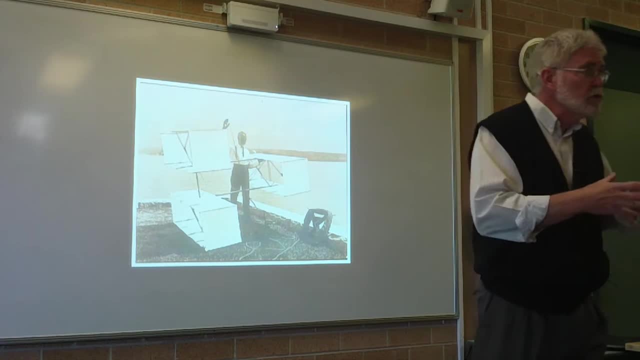 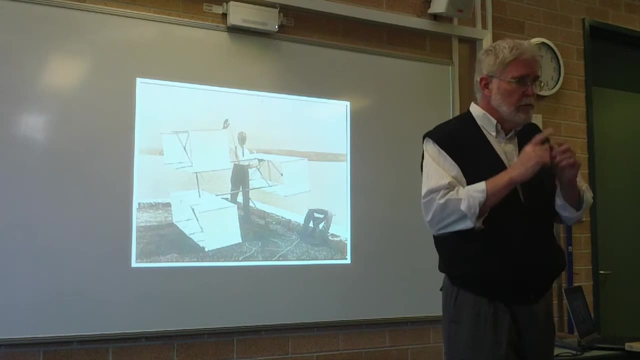 would then come into into motors. so you get all this sort and gears and and brakes that would start to be used, that would develop into other things later now- two guys actually. what happens really is that towards the end of the period of the 1900s you start to get away from big cities. didn't like having horses in the big cities. they smell, they leave deposits around that need to be cleaned up. so the bigger city started to, particularly in america, started to say: look, leave your horses at the city boundary and then you know the, ride a bike, come into town and walk and so on, and they had trolley cars and trams and other things being used. 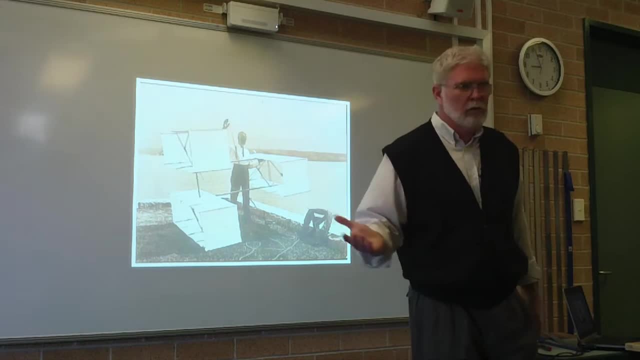 for transportation. Now they still used horse and cart right through into the 1920s and 1930s, but it was not that popular in the big cities because of the damage, not the damage, what you had to do after the horse had been through it. So it became popular to have a 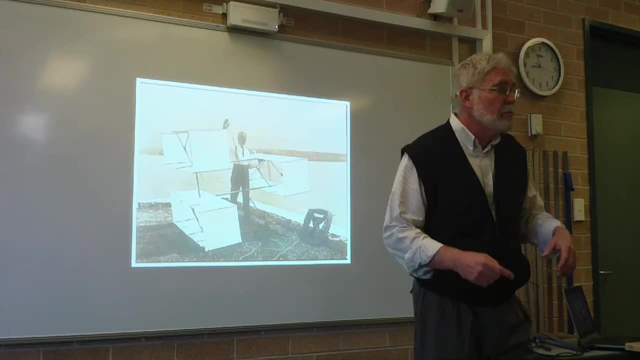 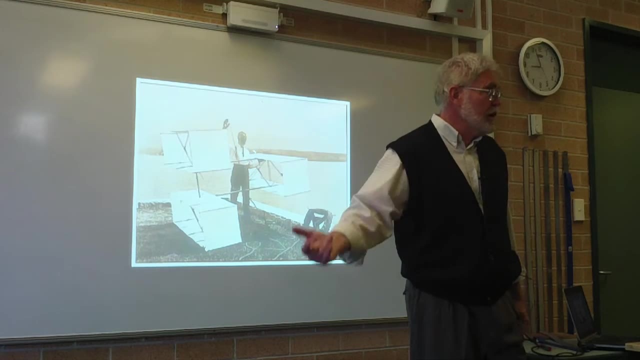 bicycle. So if you were an entrepreneur then you would set up a bicycle shop. They were very common. Bicycle shops were as common as the garages we have today- service station garages. And in a town in Illinois- you know, in Missouri or Illinois, you have to look it up- a midwest town. 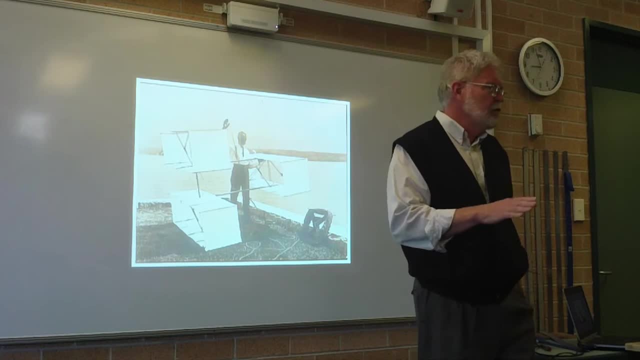 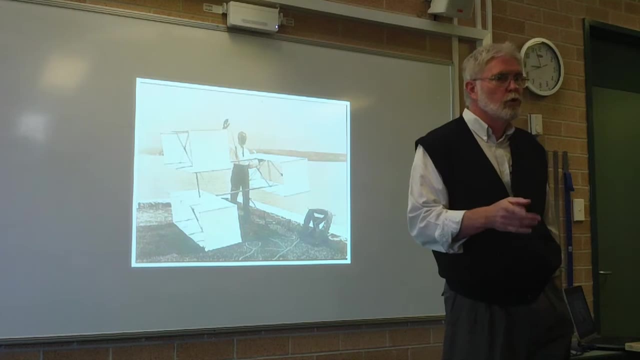 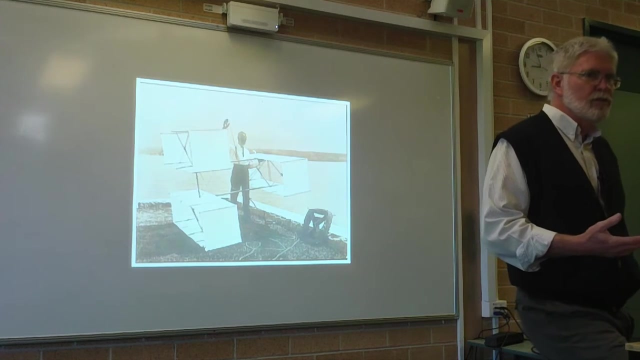 two guys, two brothers, set up a little bicycle shop and were very successful, And this is the Wright brothers: Oliver and Wilbur. Basically, what they did was that they were so successful, they had plenty of time for other things at the same time, So, and they had. 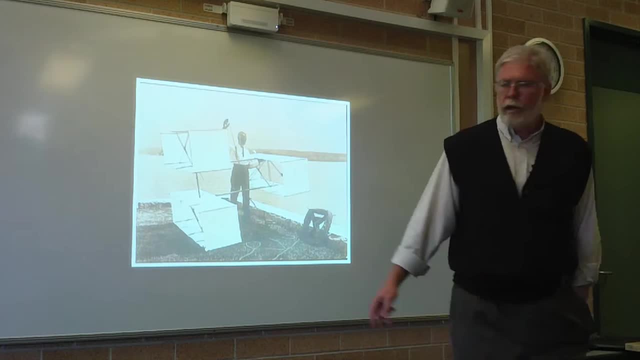 a bit of money and they were very interested in science and they had read the stories, stuff that Hargrave had done, and they read the stuff that Lilienthal had come up with- and they started to do experiments of their own. And one of the good things that they did- 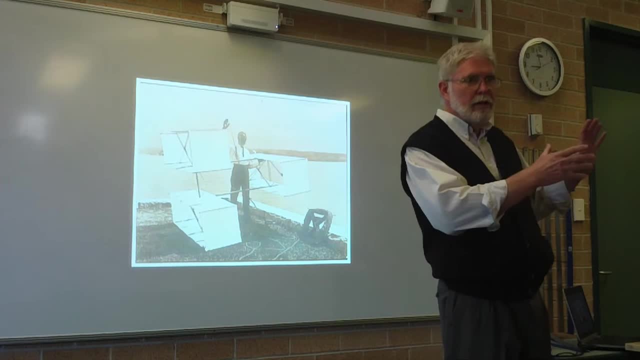 one of the things they were able to do is because they had a bicycle shop and a machine shop out the back. they built themselves a wind tunnel using bicycle pedals and stuff to generate a fan to blow wind so that they could put models of designs that they were working on into the wind tunnel and 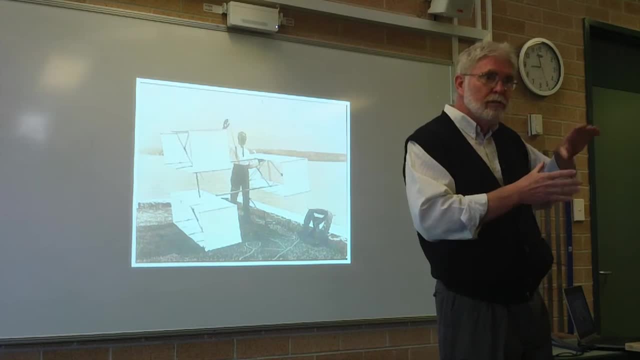 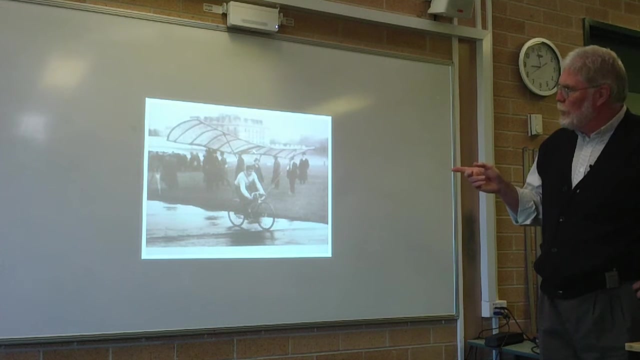 see which would lift off the ground, What sorts of wind and what speeds. And they were able to do scientific testing of designs for wings and aerofoil shapes And eventually famously- oh hang on. before I go there, I had found some slides. 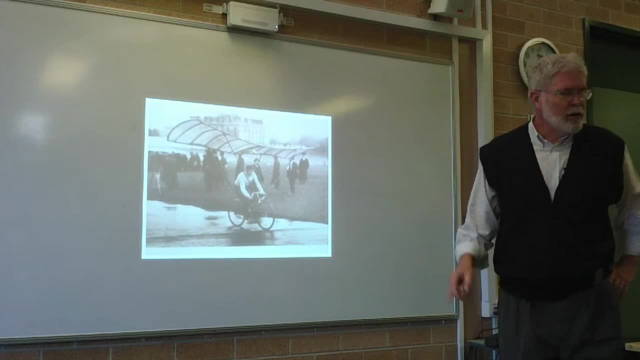 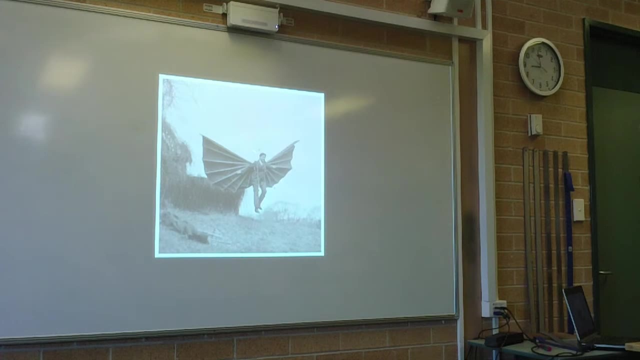 of people who were, at the same time, trying to find out how to fly. I put this one in my list as dumb, all right. and I put this one in my list as dumber, all right. This guy tried flapping, seriously. 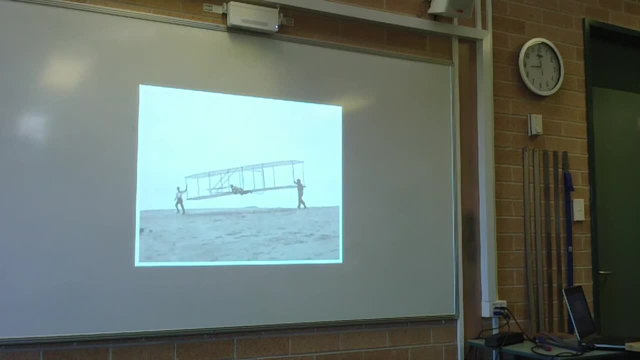 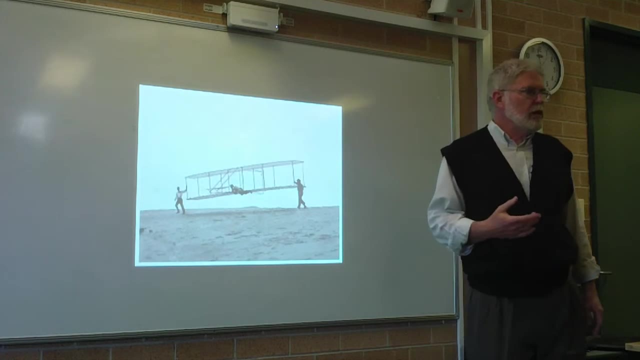 Seriously flapping, you know anyway. So get to the serious stuff. All right, The Wright brothers are famous for taking their designs out to a field of Kitty Hawk, where it was near the sea and actually near the lake, So the water, the wind was blowing off the 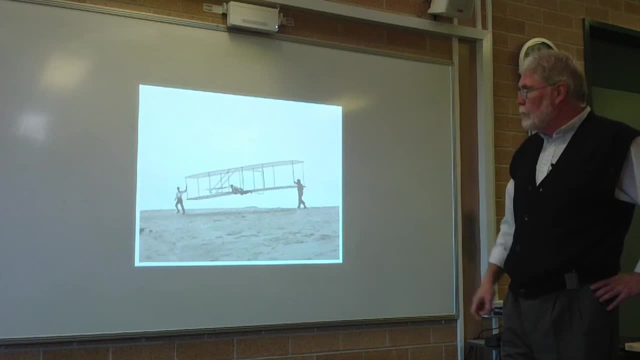 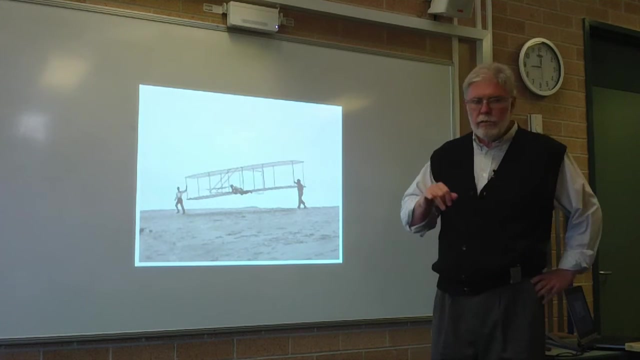 lakes up over the sand dunes, And that's a photograph of some of the testing. Now, at first it's just simply a man sitting in it, like Lilienthal's stuff, So he a hang glider. basically, The control mechanisms. that's what they wanted to come up with, control mechanisms, And they knew 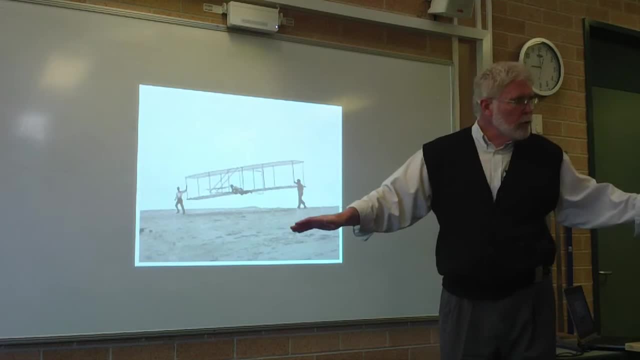 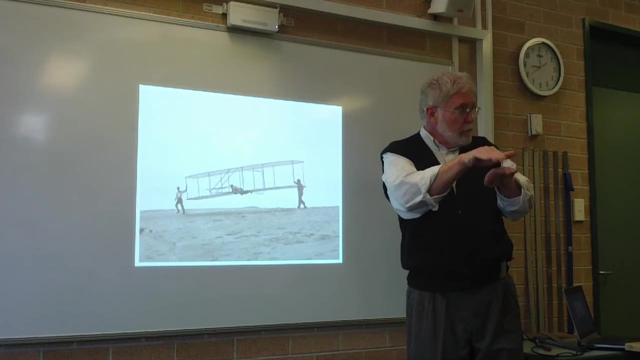 something about that. you can't just go up and hope to turn and use your body weight. So they brought in a canard wing at the front, tiny little wing at the front which could be tilted up and down to give attitude to the front of the aircraft. And they put a rudder on the back. 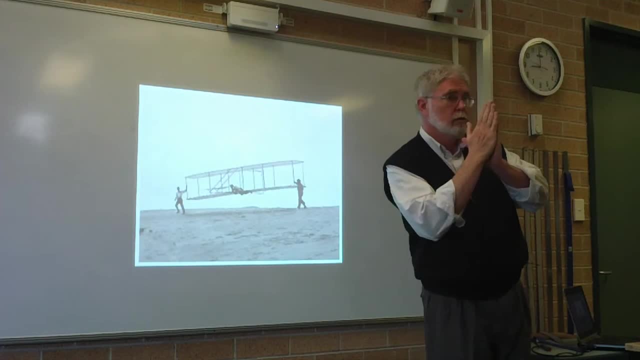 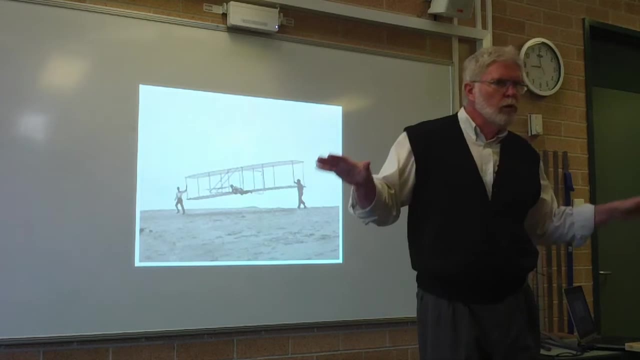 which was foot controlled, to turn into the wind so that you'd turn left or right. Now, at this stage you haven't got to the complex things that you put on the sides of the wings, the aerolons to give the wings tilting so that you can turn and bank. That would come later, but they were at least on. 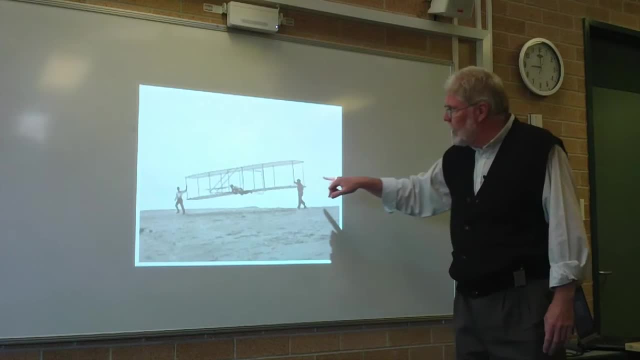 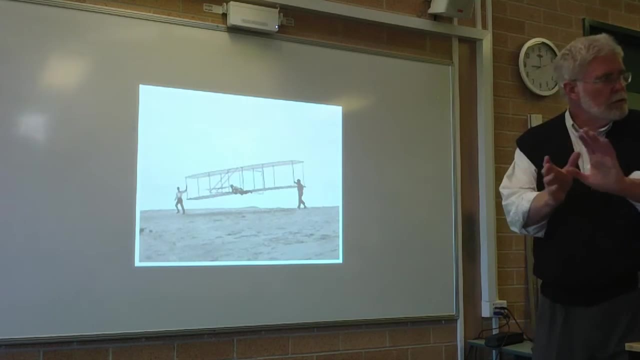 the right track. Again, pinching ideas from Hargrave. See the structure. it's very similar. So what comes before and what's thought about before leads to someone else putting it all together and coming up with the right combination at the right time. There were others. This is a. 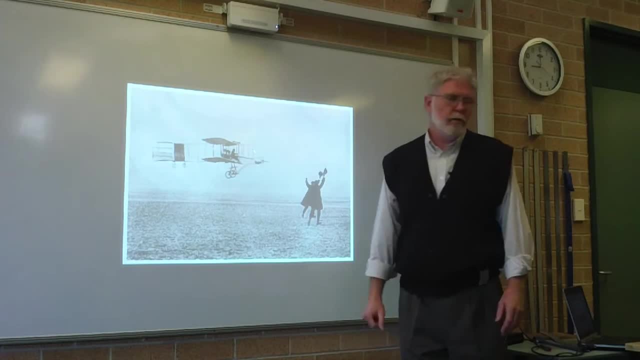 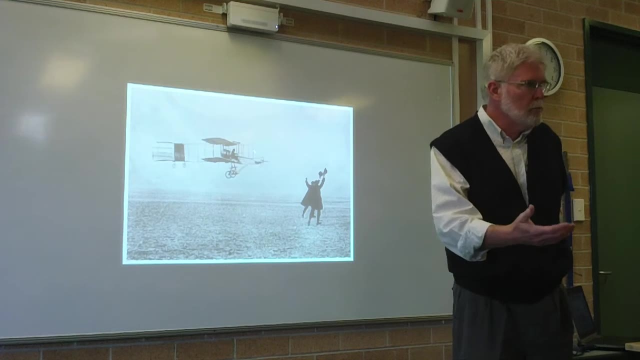 famous flight one, too, because this is the first time a powered flight is being photographed. Again, it's the Wright brothers. So this is a flight that's going to be powered and that gives you more control, because the other one is just a hang glider. You rely on the wind. 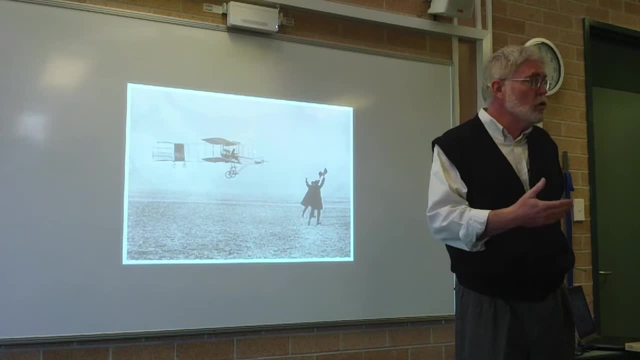 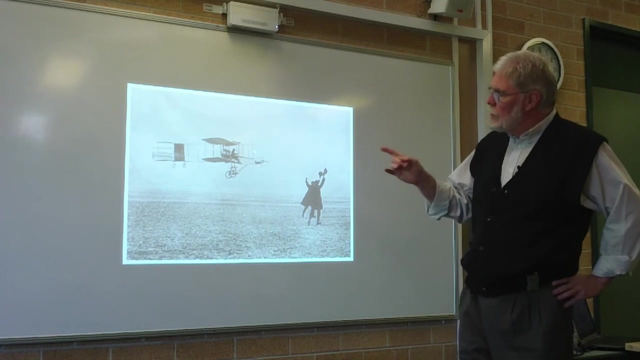 The first flight of at Kitty Hawk was no longer than the wingspan of a 747, about 300 meters. It's not really that remarkable, but when they get powered flight they could fly a lot further and more control. And the biggest test of all eventually was: could you turn and come back? 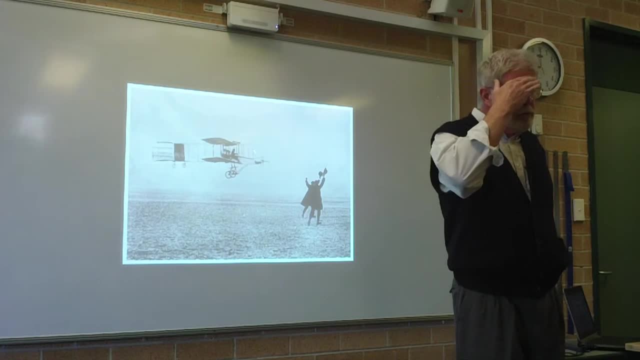 to where you started. In fact, the- I believe the- the military were very interested again because they could see the opportunities as presented here and they had a contract ready to be signed for the first person who could demonstrate control flight which included. 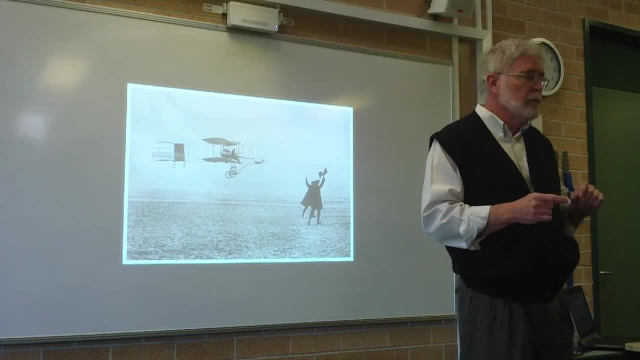 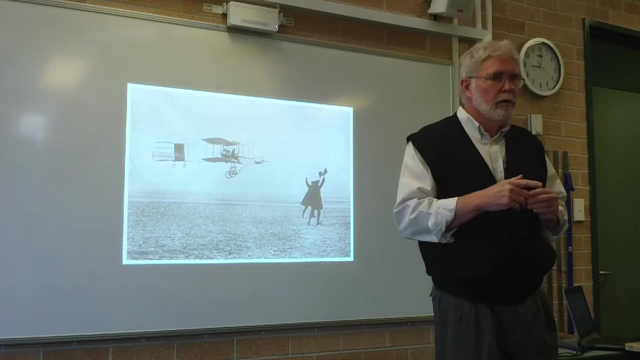 circling and circling a field and coming back and landing in the same place they left. The Wright brothers and another bloke, Curtis, were fighting out for that particular contract And there's a bit of argument: who got there first? Curtis gets the military contract and the Wright 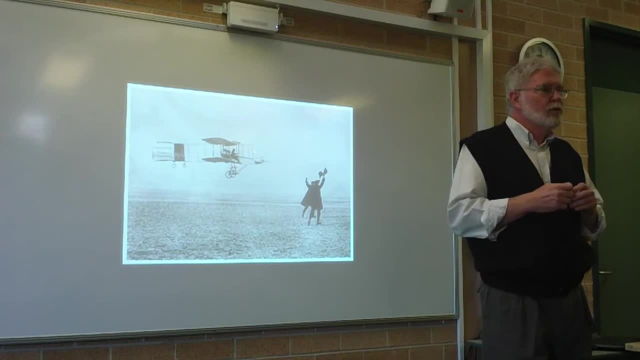 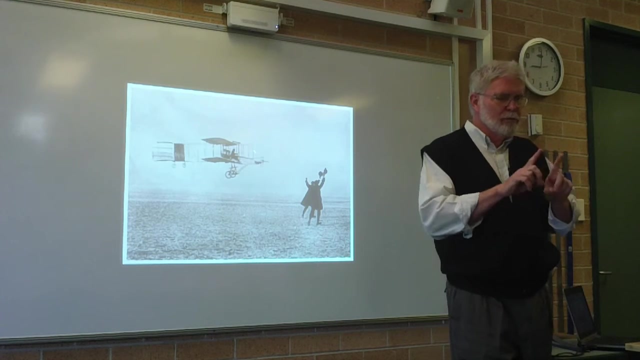 brothers are famous for being the first to fly, so a lot of Curtis aircraft were the first American military aircraft. later in World War two, you might have heard of the Curtis Kitty Hawk. all right, probably a bit of a misnomer, because I don't believe the. from what I've heard, the Wright brothers and Curtis got on. 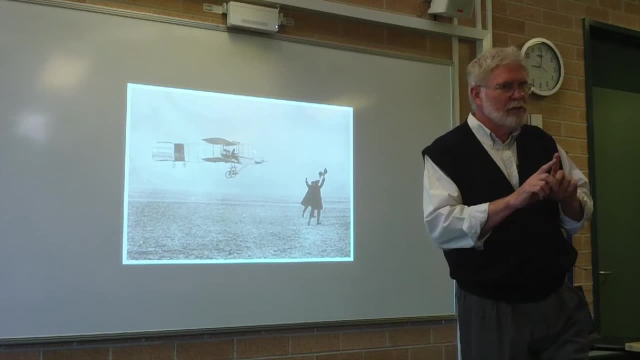 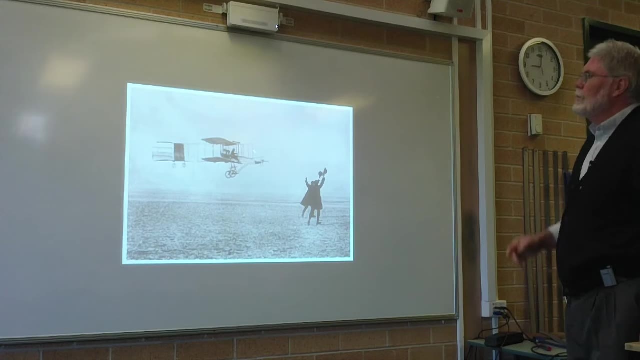 very well so. but that suggested if he named one of his aircraft or allowed one of his aircraft to be named after the field in which they first fly, flew, he may have been paying homage anyway. so the principle, the things that were in the planes were there from the first bit. there's that Kennard thing. again the 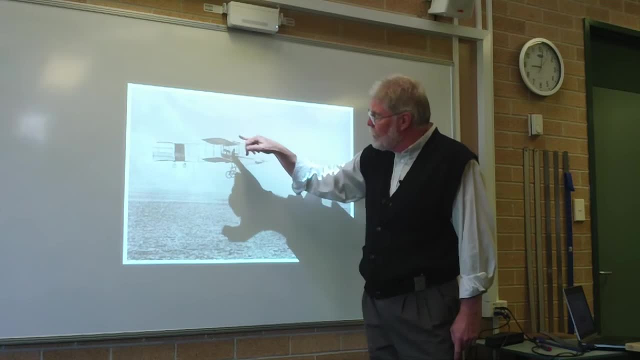 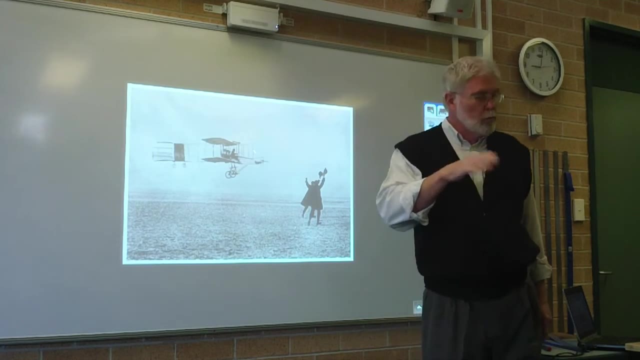 structure is a compressive structure. you've got your airfoil shape, which we'll talk about in a minute, and you've got a rudder, so certain things that were familiar to aircraft or will be familiar to all aircraft from that point on. but the big deal about the motor is that you first needed something light that would 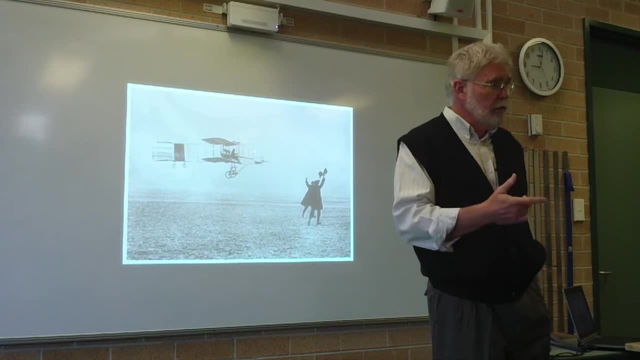 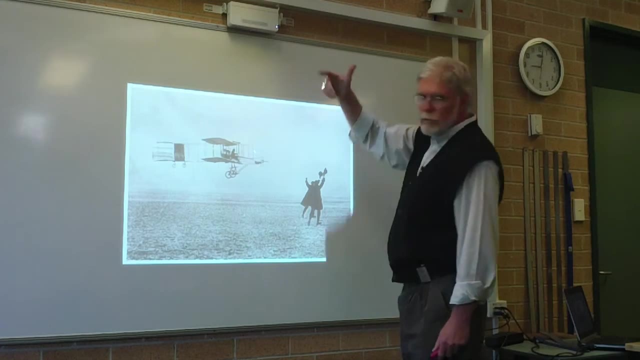 produce the aircraft, and that's what the Wright brothers did, and that's what we were going to talk about in a minute now. the second thing is that you need to produce enough power to get you to get to the lift position. now what I might do is just change the setting here for a minute- where's the thing here? and go to 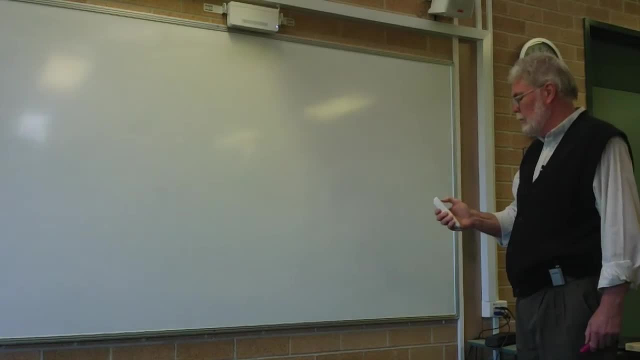 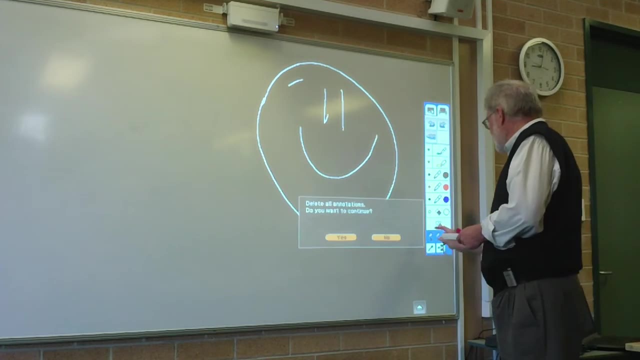 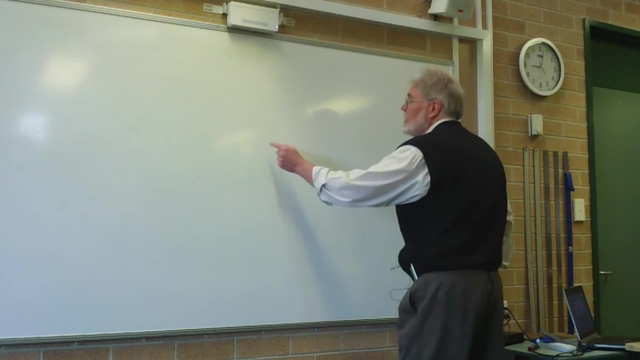 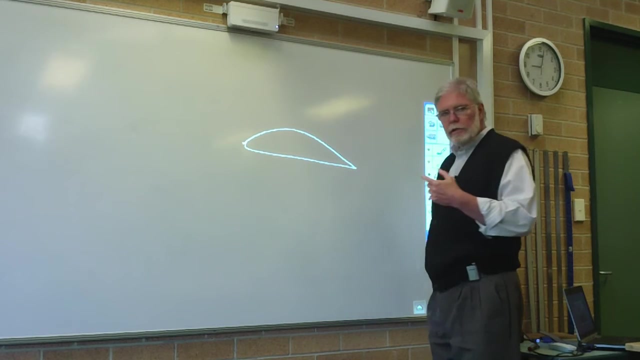 the board because I want to talk very quickly about where are we. so, if we go USB, no, it's not that, no, we just go to here, that's right. yeah, I can do it with my finger, a wing that you are familiar with, known as an airfoil. basically, the principle here is something that we're going to be talking. 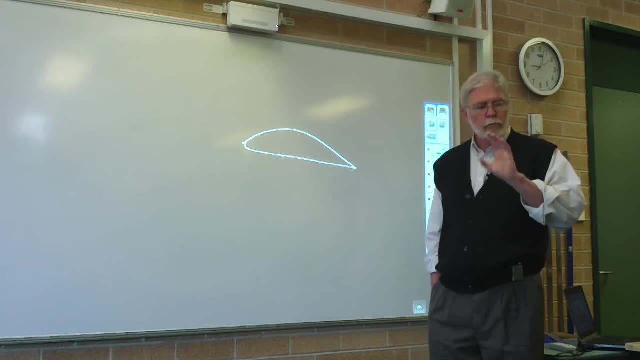 about at length because we need to look at it from the detail of how we came to that, and we're going to go back in a moment to another scientist from the 16th- 17th century who did give us the information about how this works now. 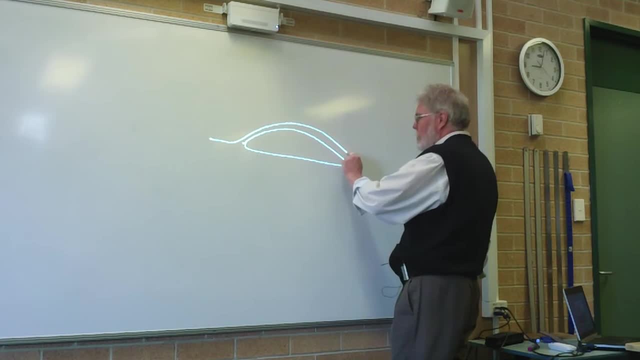 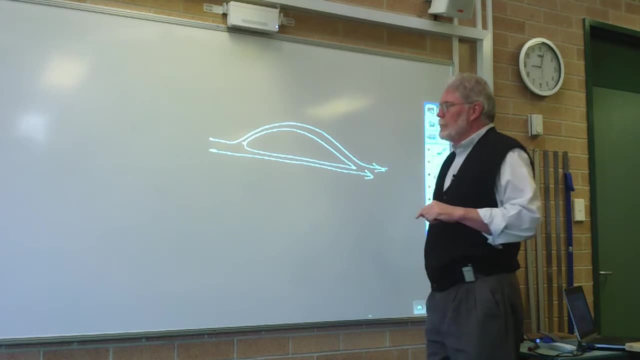 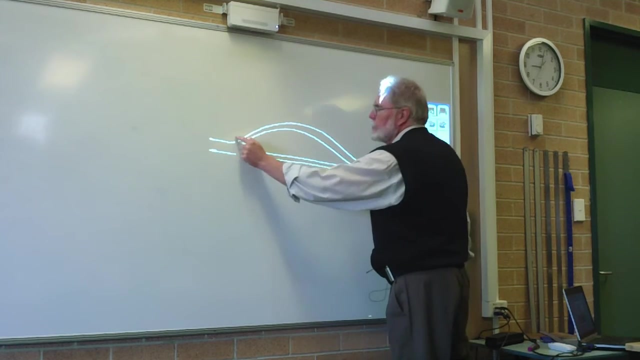 basically what happens is the air flows over the top and comes in at the back and meets the air that's coming underneath, just like that. but it's quite clear that the distance traveled by the air going underneath compared to that traveled by that over the top very different. now the 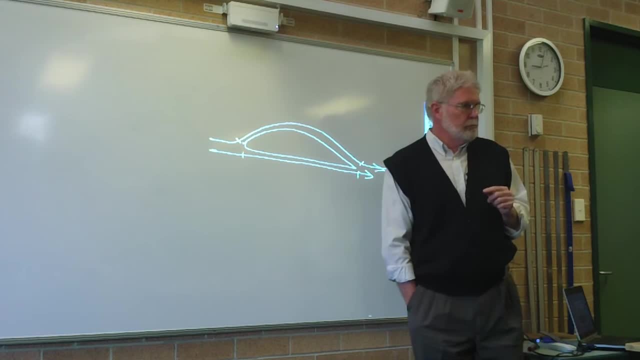 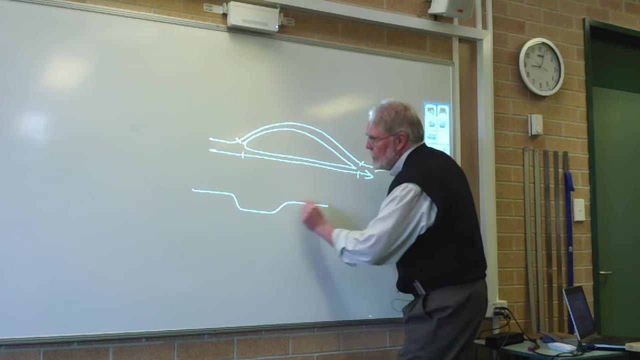 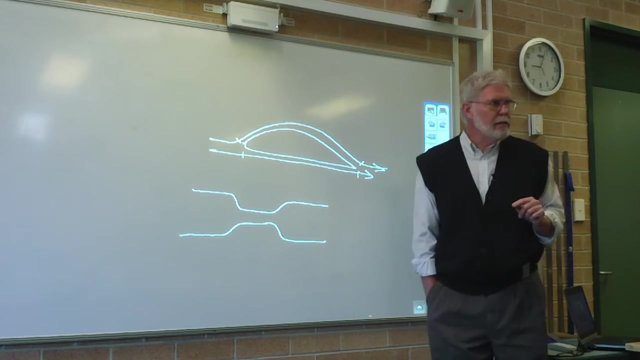 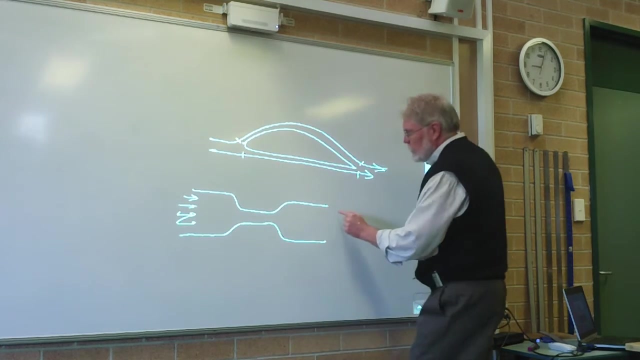 principle that's applied here is Berlin's principle, and he did as an experiment, in which he noted that if you have a pipe that has the same shape as on the outward side as it has on the inward side, but you squeeze it in the middle and you put into this end fluid and you allow the fluid come in and out. 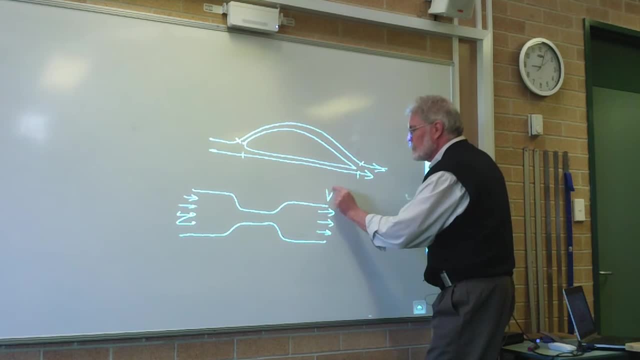 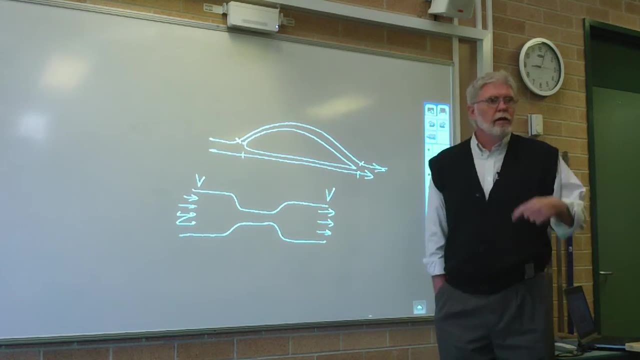 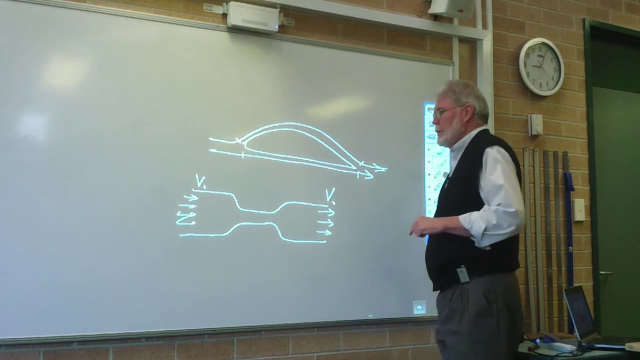 at the same rate. so the velocity of the water coming out here and the velocity of the water coming out here, or the volume of water coming out at both ends is the same. so they're equal. so let's say: velocity one, velocity one. what he was intrigued by was that. what does that mean about the? 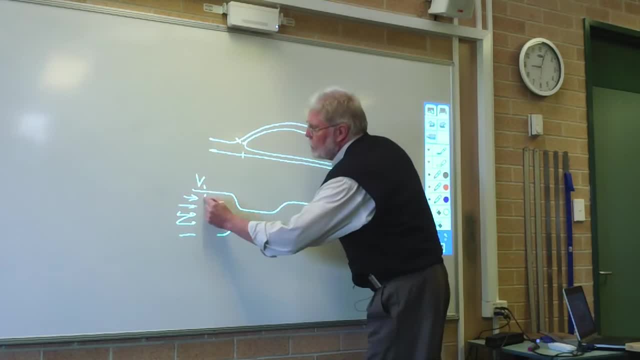 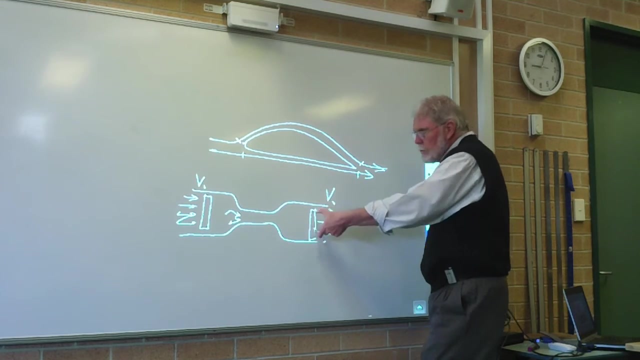 fluid going through here then because if you've got up, say, a section of fluid that big a volume of fluid, when it gets to here it's got a squeeze through but it has to leave at the same volume. so this amount of water and this amount of 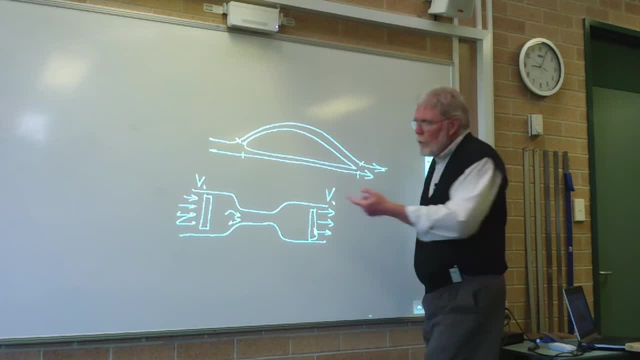 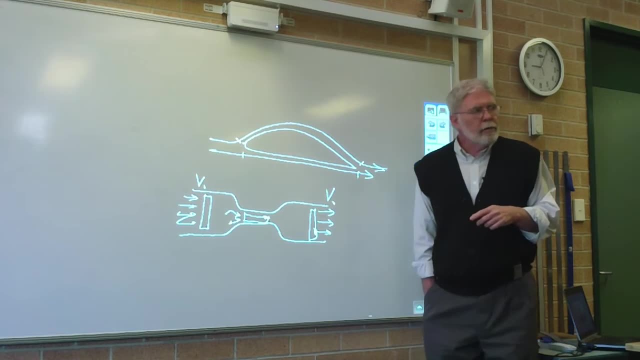 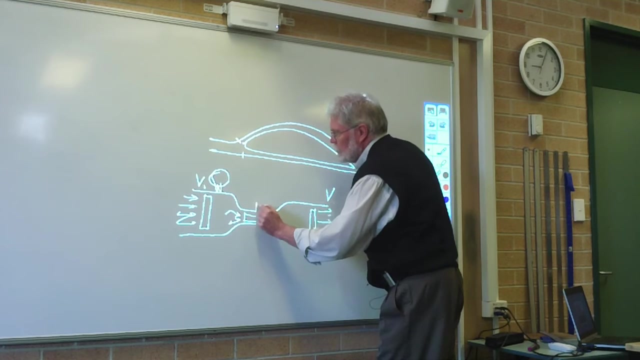 water comes out at the same time as coming in, so that amount of water has to squeeze through here and arrive out here quick enough to come out. so what he found out- and he did this by checking the pressure- put a little gauge on here, gauge on here and a gauge here, and he noticed that the pressure on here. 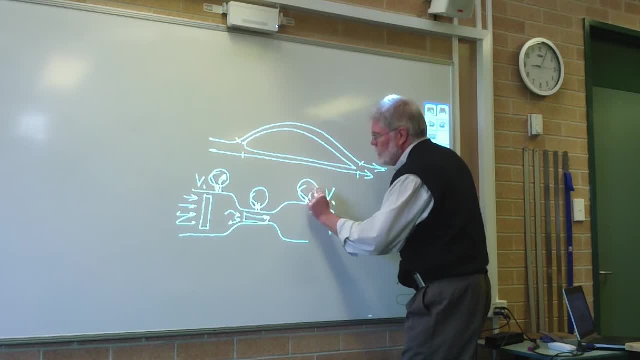 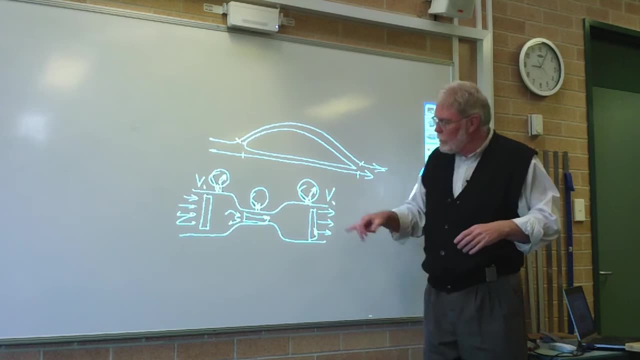 might have been registering over there, pressure over here. now, pressure is related to the volume and the volume which is pushing on the sides of the container and so it's moving through the container out. so the it's logical that if this is traveling at the same velocity, same 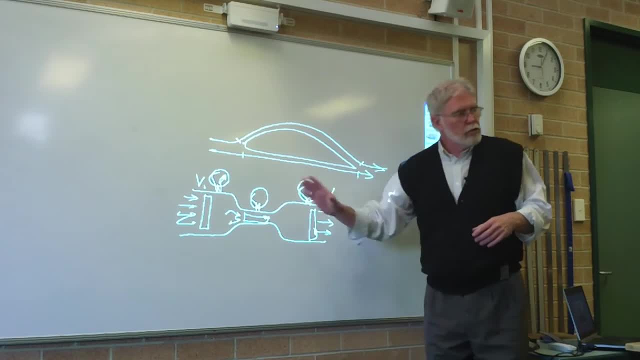 amount of water coming in here, same amount of water going out here. you'd expect the pressures to be the same at any point in the pipe, so what he noticed, though, is here pressure went down and the speed went up, so this was a new velocity, and that makes sense, because if you've got one or two particles of water, 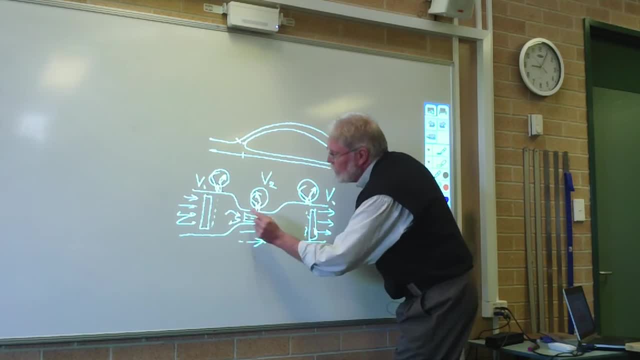 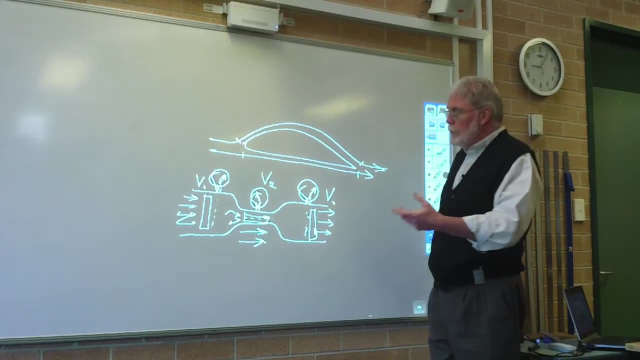 here and you want one or two coming through here, then they have to come through here quick to catch up with the ones that have already gone through, so they spread out. that's important. Bellini's principle applies to this by saying: well, as the air goes over the top, the relative density of the air spreads. 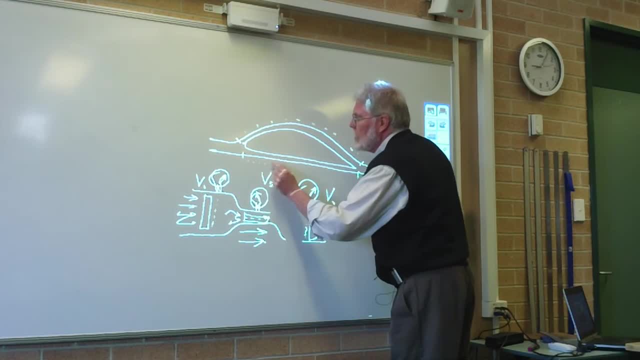 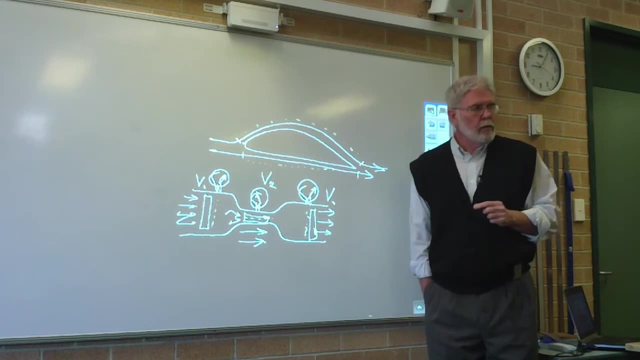 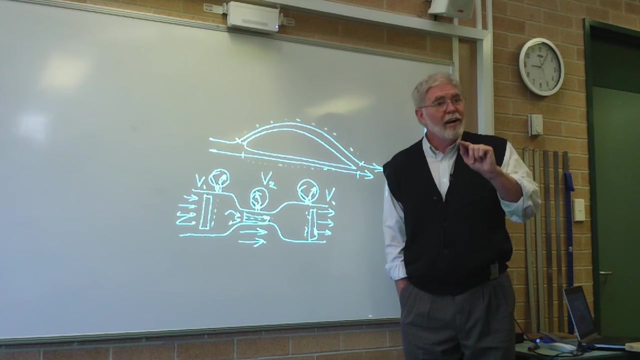 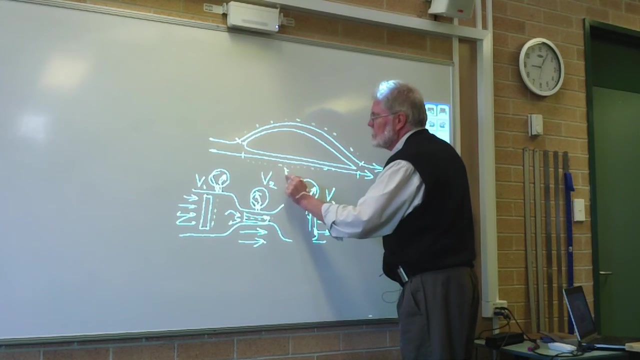 out, whereas coming underneath here to keep the same number of volumes coming through, the spacing between the molecules in the air stays similar all the way along. that means the density here is higher than the density above. the pressure is higher. it is lower above than it is below. so here's the principle. here you've got one set at one pressure. 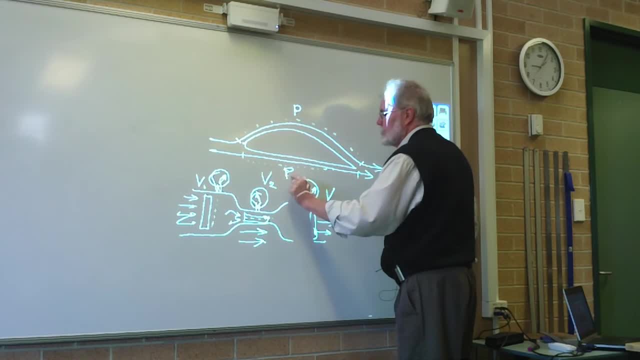 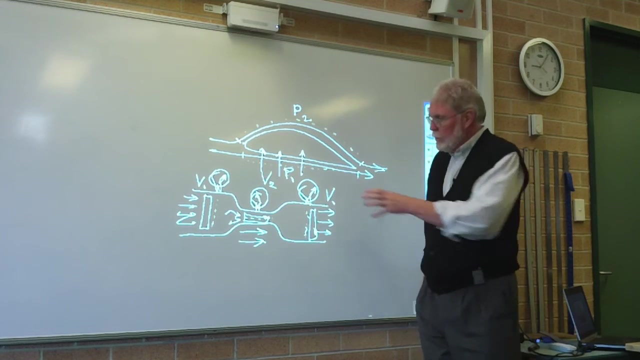 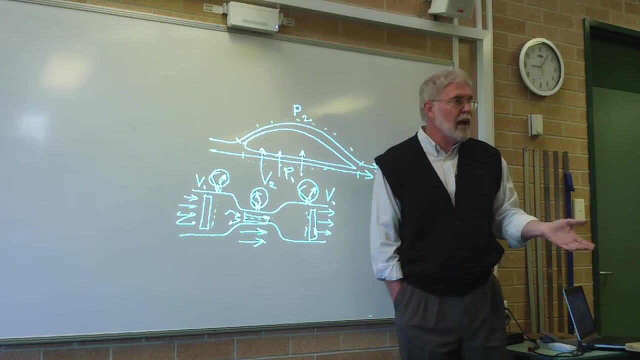 and here you've got a lower pressure. pressure one, pressure two, because this is lower. the air spread out. this guy pushes up its buoyancy again at work. that's flight. the Bellini principle applied to an aerofoil. now it takes them until the late 1800s, not late 1900s, to work that out, of course, and that's what really was. 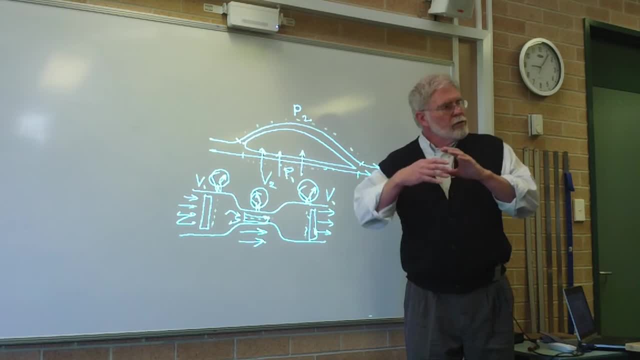 being done by Lilienthal? really, what was behind Hargrave's ideas with kites? Hargrave was working on the idea that if you had a kite box kite, one of the reasons it flew was, as the air went round, it created a partial vacuum behind. 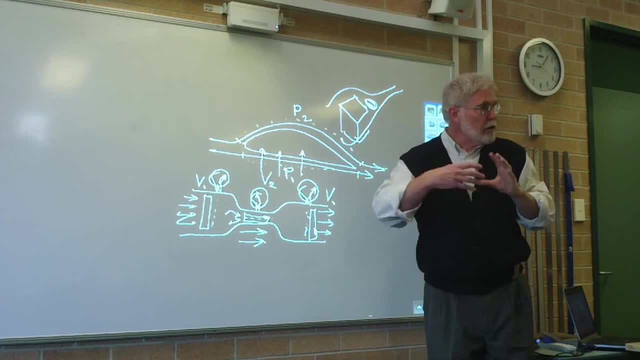 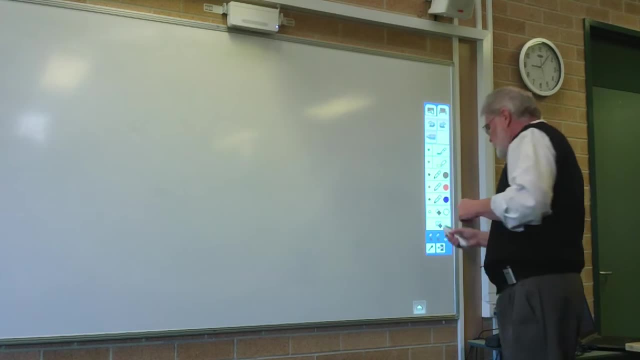 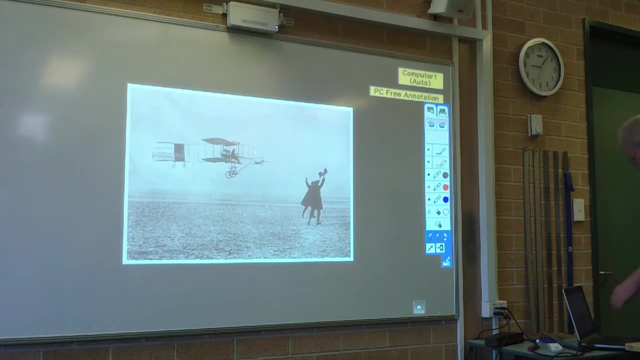 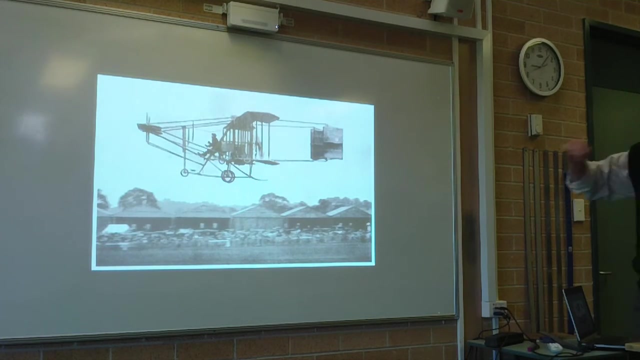 and that vacuum would draw onto it. so he worked out the box. kite shape worked better anyway. so let's go out of there and go back to our slideshow, which was on computer. so there you go, we're at these first flights. what do you think is important? that comes next. oh, by the way, just here, this is. this is a better. 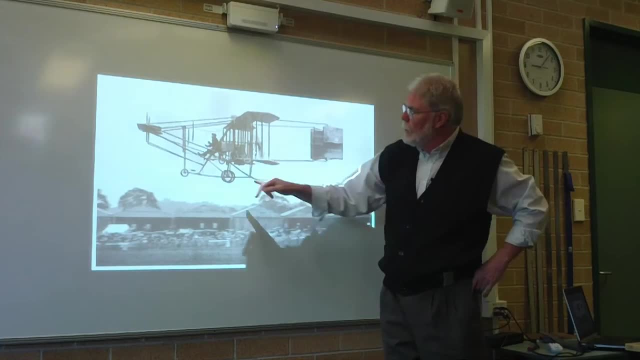 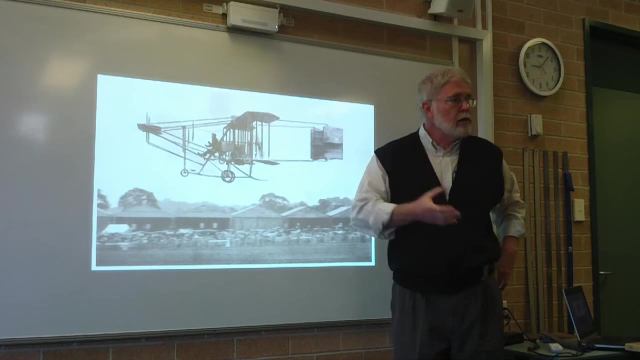 picture showing all of the main things from an engineering perspective. you've got bicycle wheels really just being used. the framing is just tubular or wood. actually it's mainly just made out of timber. that's been because timbers lighter than metal, so therefore you use your timber the the wing. 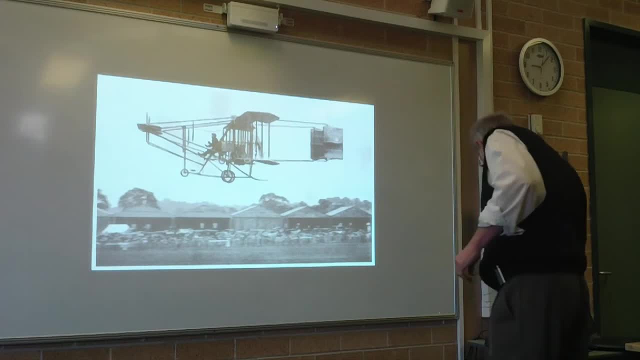 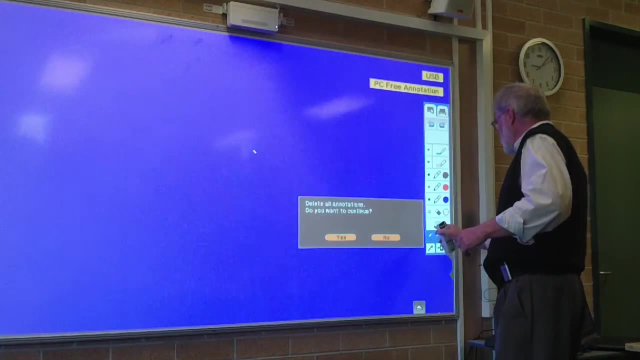 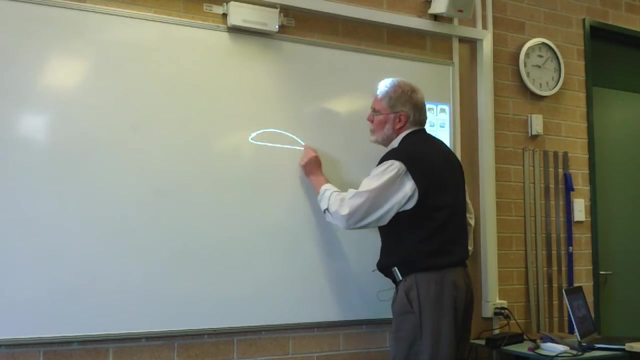 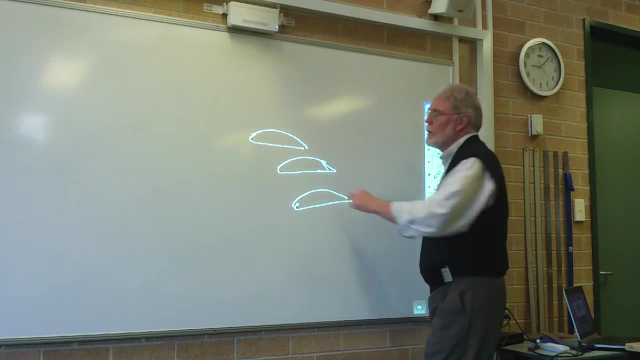 structures, wing structures, in those days- I'll probably go back again just for a moment- what you did was you built your aerofoil into a series of wooden pieces, connected them with spars- thin pieces of wood, one on the bottom, one on the top, and then, to keep the light weight to it, you would cover it. 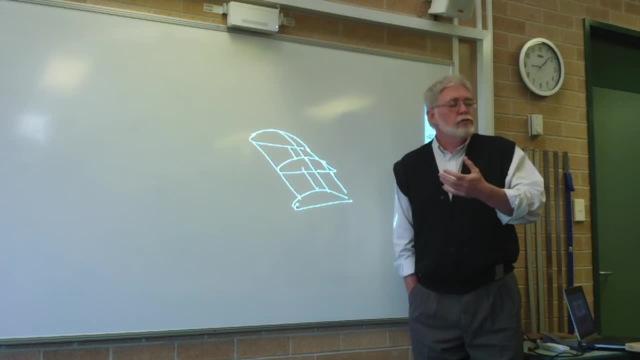 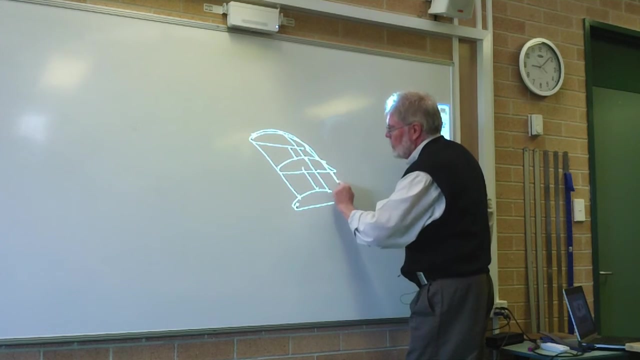 with a very thin material, perhaps a canvas, or even, as the Germans would later do, put on a paper, very heavy gauge paper, and then paint it with a resin material which would would shrink when it dries, so the shrinking would tighten over the surface and create a thin layer of material covering the whole thing, and 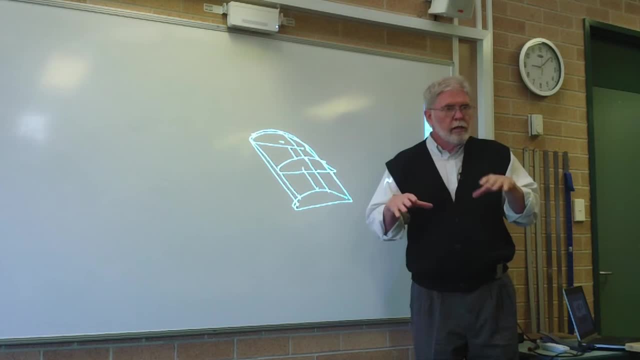 you got a very lightweight shape. when we go to the Air Museum and we go and have a look at the stop with camel that's there, they have a section of the wing that you can see into and you can see how thin the walls are and basically the 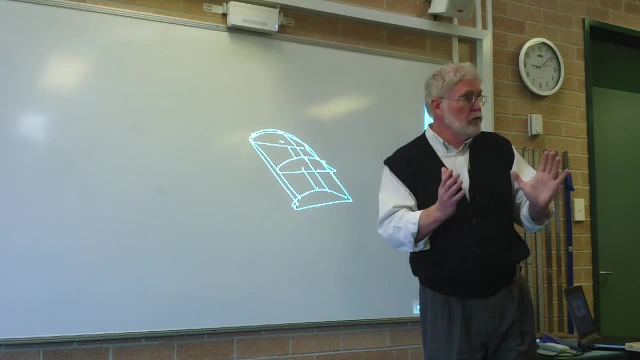 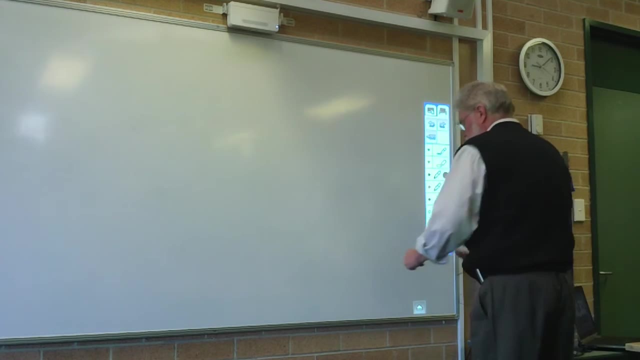 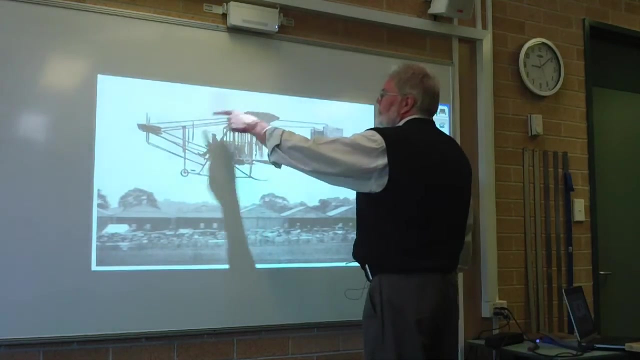 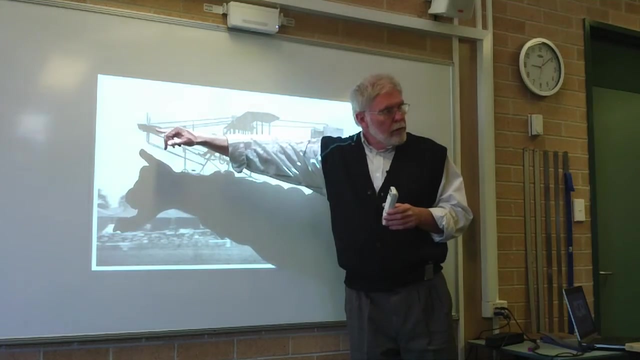 whole aircraft is just covered with this doped material, the textile material. it's taped on the outside, back to the other thing. so they always do this right. that is your general shape. that starts the plane. but here's the big difference today: that particular control mechanism at the 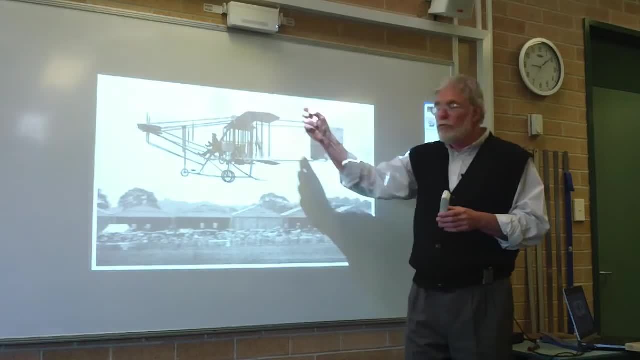 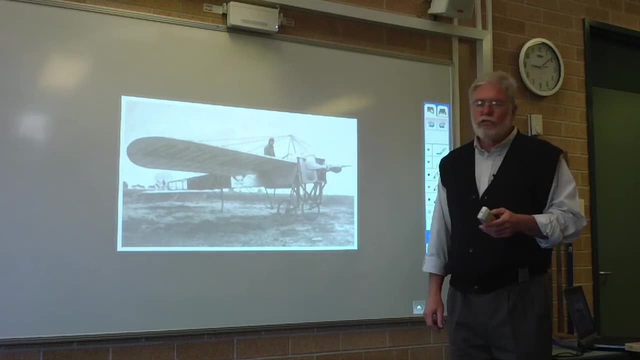 front. the canard at the front gets shifted to the back and you start to get a plane shape that you're familiar with. there's your standard sort of I'd know that's an aircraft anywhere. you've got your big motor thing at the front here which occupies the majority of the plane, and then you've got a little bit more. 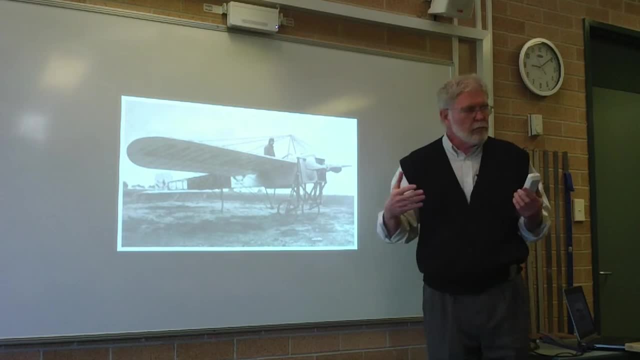 of the shape you. so you put your pilot behind that because he's got to get out of the road of the wind. so you create a fuselage that allows you to get your rudder and flaps at the back tail planes that can be used like the front canard. 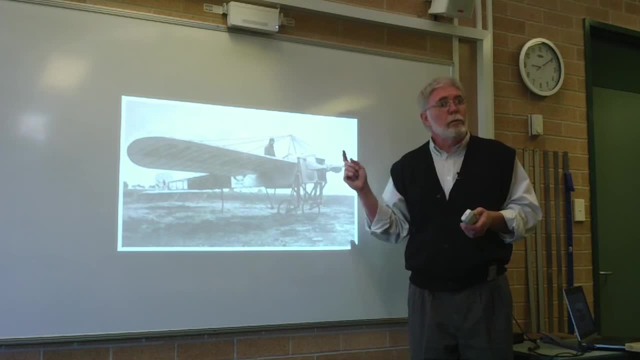 the difference with the Wright brothers. one was that the propeller faced the backwards and pushed the air. this one, it's turning and dragging the air. air screws, by the way, are worth thinking about by themselves, propellers, because that's a technology, technology, that's a technology. that's a technology that's. 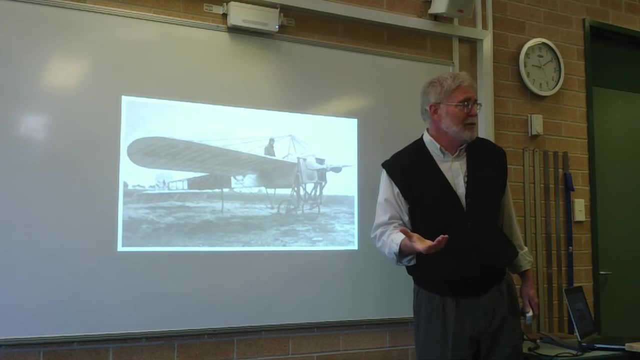 you had to get from somewhere. so where do you think they got it? from ships. it's nothing more than realizing that the air can be dragged, just like a ship can pull itself through the water. now notice, here we've got some structural elements that are taking place that are interesting. the wings have clear aerofoil shaping to. 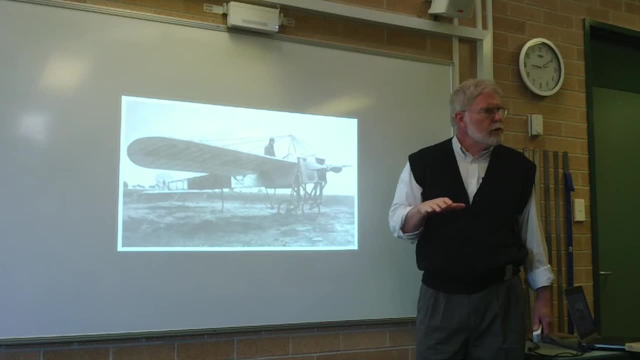 them not as great. they actually tried to trap air under some of these two. so you've got this scooping effect. later on they'd realize that you actually don't need that and they'd straighten out the bottom of the wing. but what do you think? 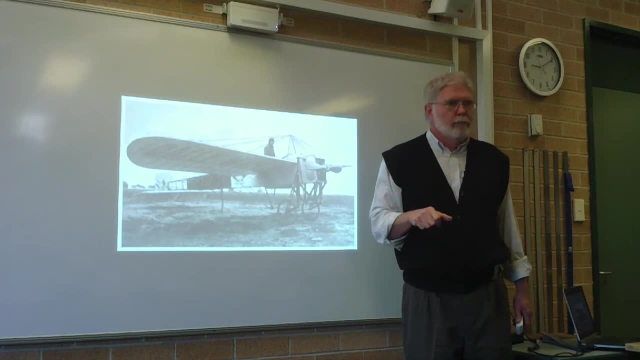 they're doing here with all this wiring right, because what sort of a shape do we know that wing to be if it's sitting out there like that? the term we use for beams and things canter lever right, so there's a whole lot of force on the. 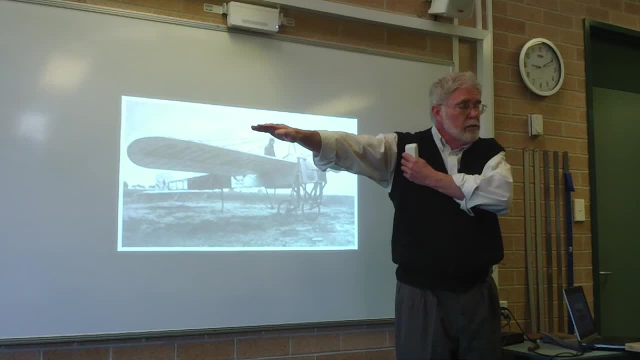 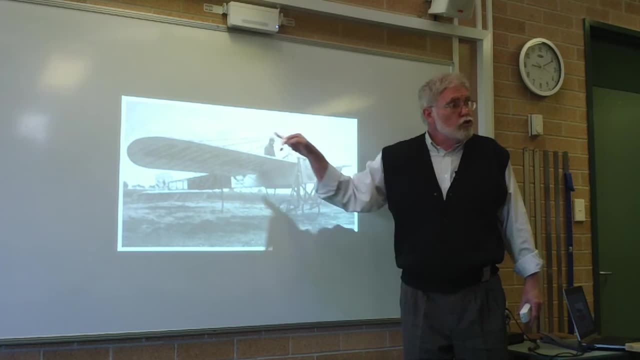 structure at this point bending forces taking place. so if you tighten the ends up on both sides and pull them towards, you really do have basically a suspension structure with the levers involved. you think, in terms of a bridge, could be built like that. not a lot of them were. all right, we've got a few minutes. don't pack up yet. don't pack up. 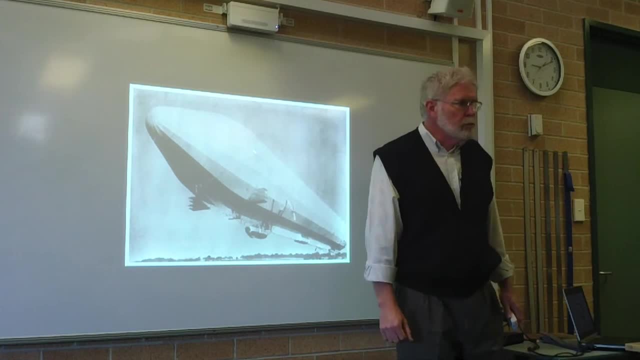 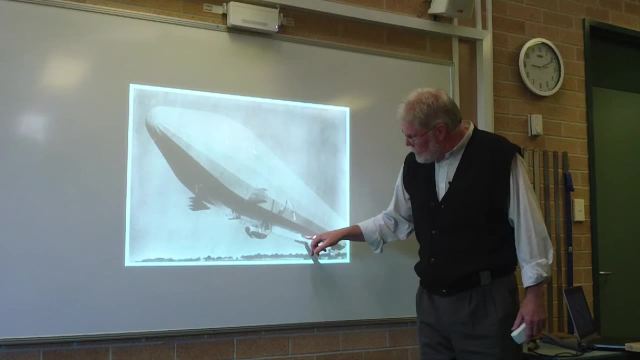 at the same time, the idea of the balloon got really big and these ships, airships, they're huge underneath here, these gondolas that fitted underneath here they the one of the Zeppelins that lie the Atlantic trade during the the late 20s, the 20s, and that were so big that they had grand. 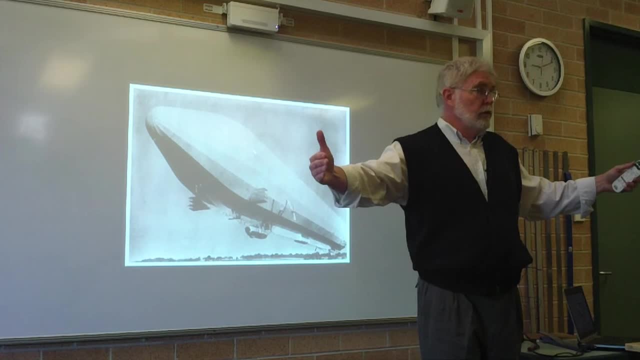 pianos in the rooms underneath this room here would probably fit into one of those things for just where people would come and have dinner and sit and they had State rooms and they had all this sort of stuff underneath, because they also built them up into the infrastructure, because there was. 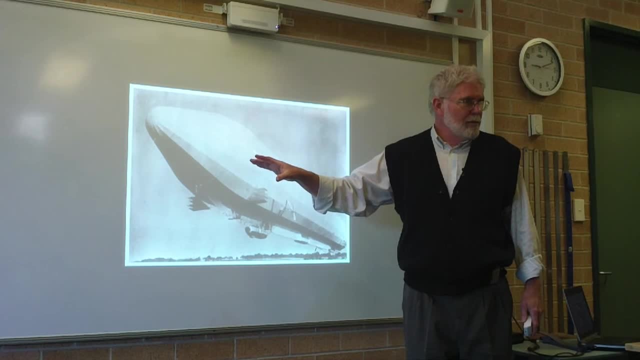 plenty of room. it's full of hydrogen and I mentioned before hydrogen is problematic because if you get a spark near hydrogen in the, in the Adelaide subcontractor, those similar things- if you have a very long form somewhere where you can get an air. firstly, if you have a very long form. 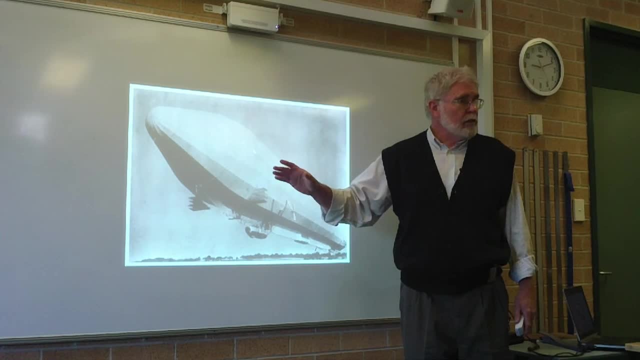 would get an air. firstly, there's a lot of air in the Adelaide subcontractor, so you need a lot of air. if you're oxygen in the air, you get a disaster out of that, and the famous one, of course, is the Zeppelin blowing up in the 30s, early 30s, the Hindenburg rather. yeah, that's. 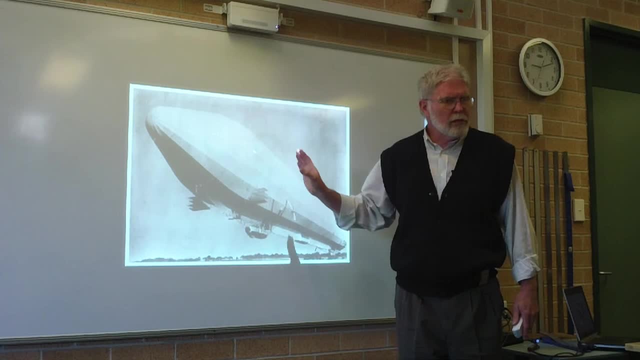 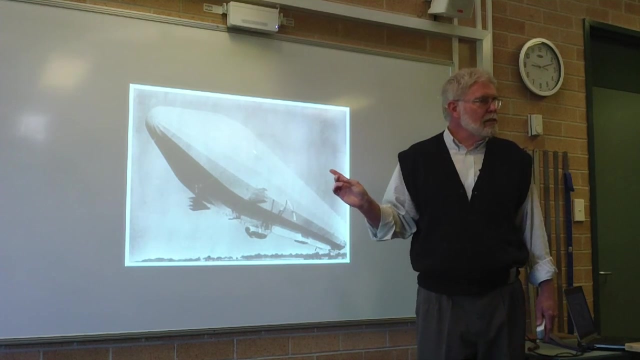 the one, and people got really disappointed with that sort of flight stuff after that. but the Americans used helium because they had a supply of helium. a lot of Germany didn't have supplies of helium. they had to use hydrogen because that's all they had. and we still use that today because you've 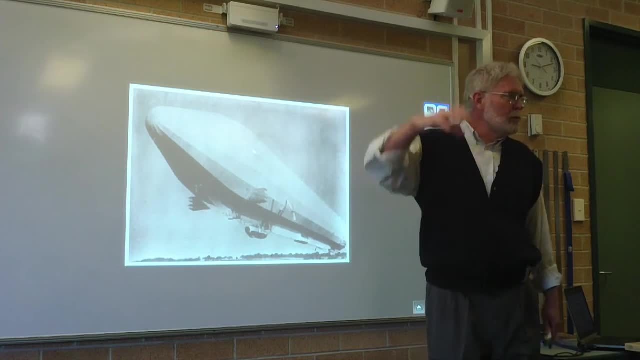 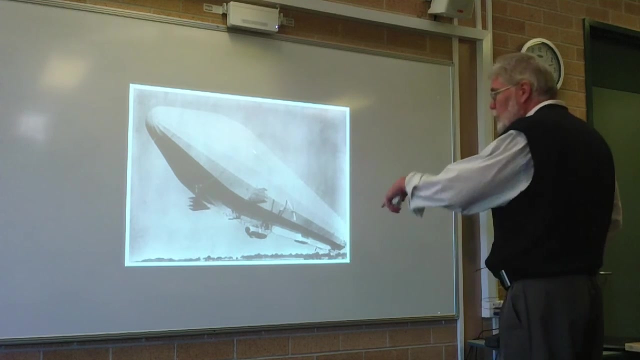 watched a sporting event, you probably have seen the balloons being used, and we still do them everywhere, so it's still a very popular means of flight. I personally would love to fly with one of those because I think it'd be really sedate, and it's just unfortunate that they they had such disasters, otherwise now we 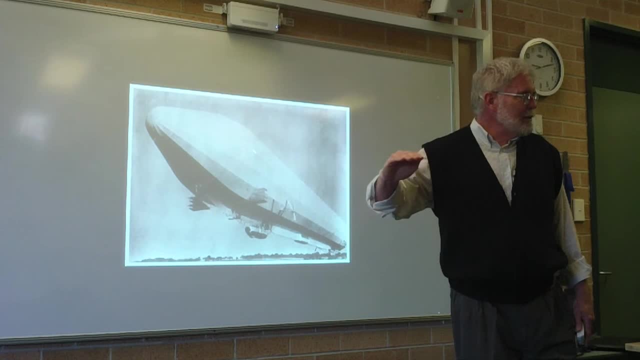 probably would be doing very sedate trips across the Atlantic, not this. I have to be there in three hours, all crammed into a tiny little seat that we can't move around in, you know, unless you can afford to go up the business class or something like that. so 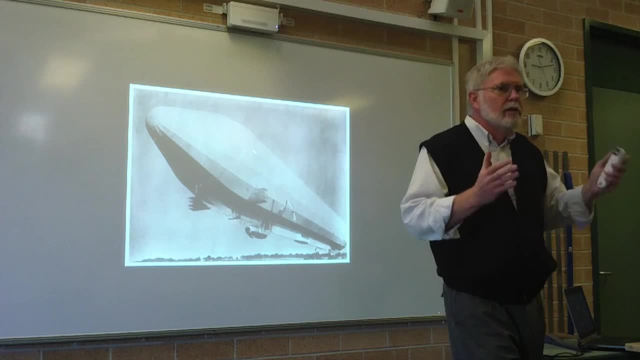 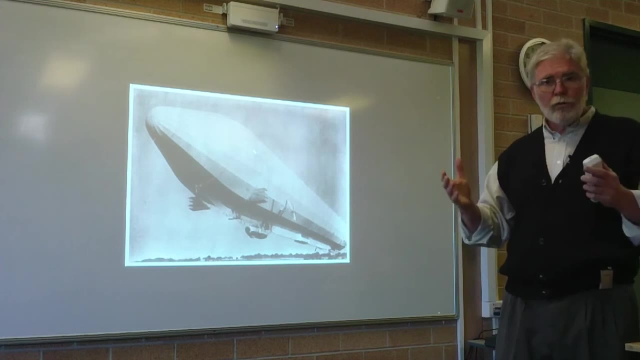 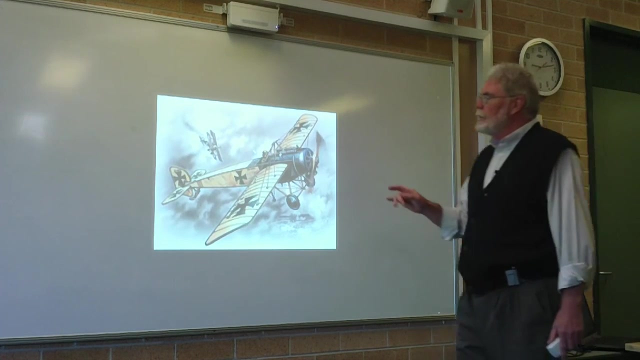 to get to make it affordable for everybody to fly, you have to put a lot of people in a very scrunched up areas. this would have been wonderful. you could walk around people playing pianos, you can go to the bar, all that sort of stuff. okay, we're going to pick up from here in the next one. 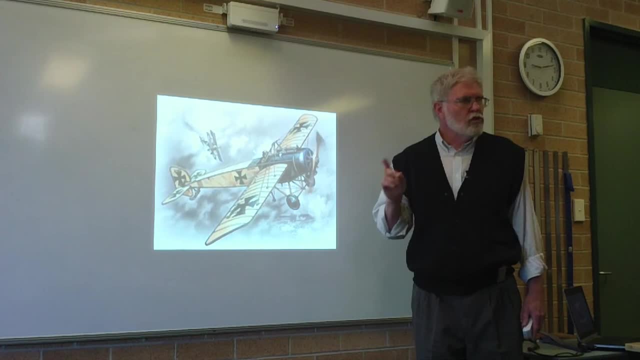 World War one, right. what changes everything is the adaption of the military to the military, and now we can talk about the military for a little bit more. but I want to talk about two military purposes now. believe it or not, they weren't thought of as being fighters straight up. the first thing: 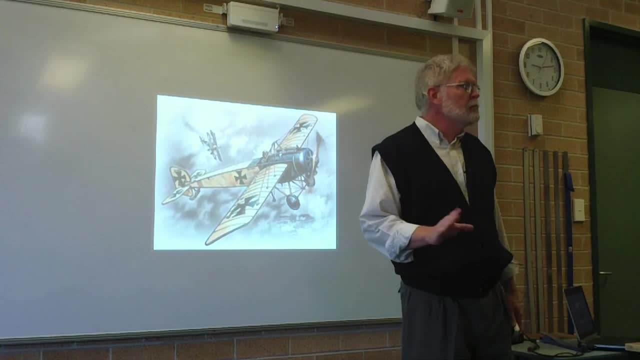 that they thought of using them for was simply reconnaissance. it was all very calm. we go up, we take some photographs with the new ideas of cameras- right, new technology cameras. we bring it back. we can show our generals the displacement, and when we take a photo, we can show what we've seen in the last few months.